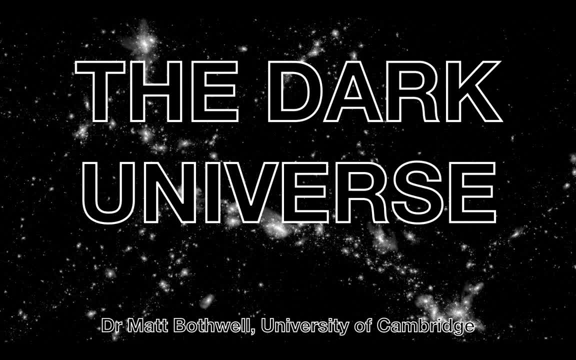 this is going to be an interactive astronomy talk. So it's going to be interactive in two ways. So you guys are going to have the chance to ask me some questions and I'm going to be quizzing you as we go along and testing your astronomy knowledge. So the way this is going to work, 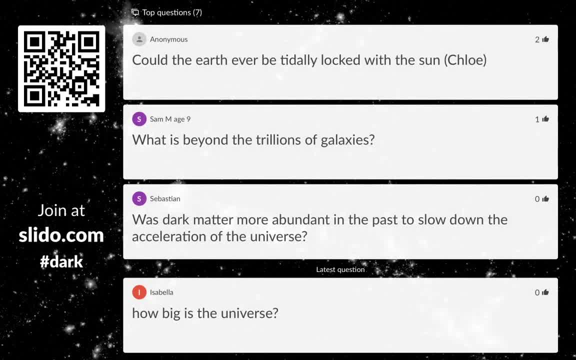 as always, we are going to be using Slido and I can see some questions coming in already, which is absolutely amazing. So the way you can join in the conversation is go to slidocom, So with a phone or some kind of internet device type in slidocom and use the. 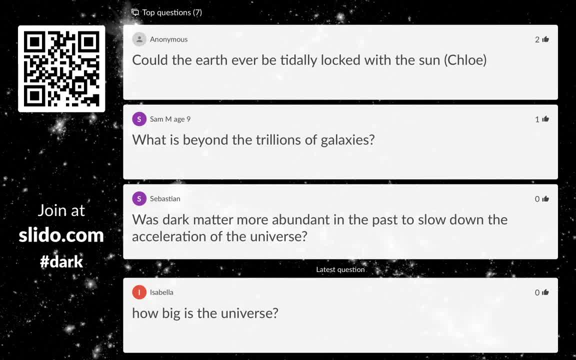 code dark or even easier to scan that handy QR code in the top left hand corner and that way you can join the conversation So you can participate in the couple of quizzes that we're going to be doing as we go along. but, more importantly, you can ask me some questions, as these people are doing. 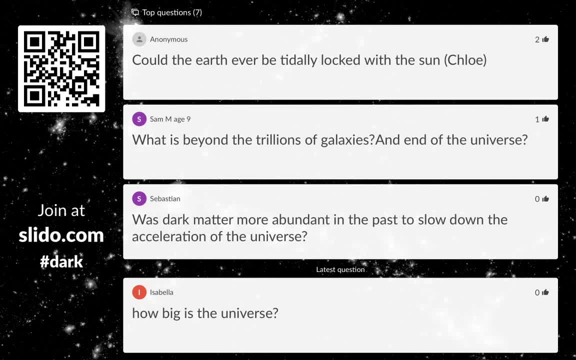 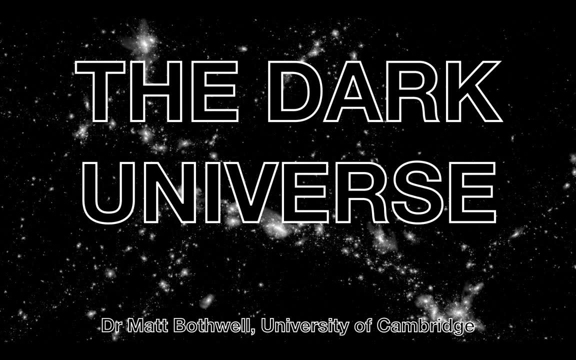 already, and then at the end of the talk there's going to be a question and answer session where all of your dark matter, dark astronomy questions that come up as we go along. So, like I said, this is the dark universe, one of the most exciting things in astronomy for me. 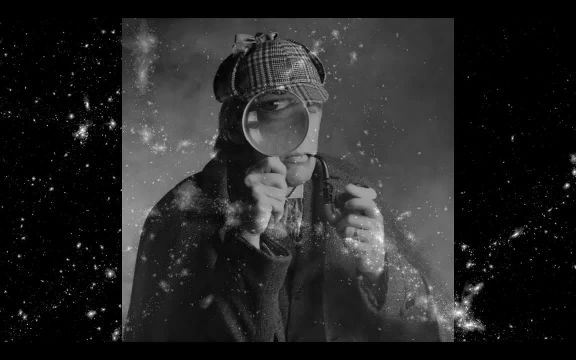 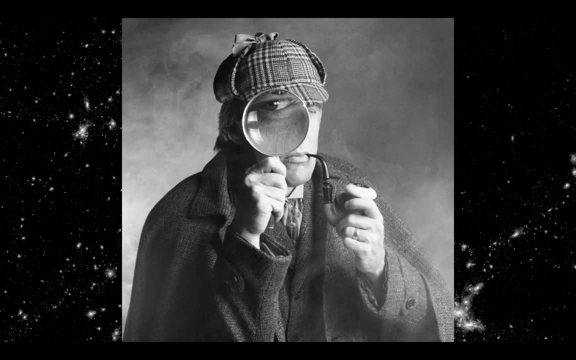 definitely one of the most interesting topics that I know of, and it's going to be something of a scientific detective story, because, if you think about it, being a detective is really what being a scientist is all about. right, as a scientist, it's your job to find mysteries in the universe, and 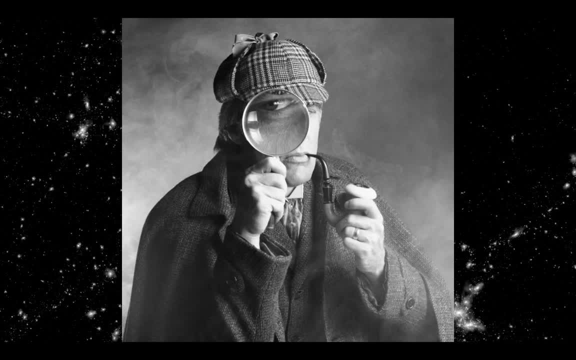 find clues to solve these mysteries, and so, when you're an astronomer, what you have to do is you have to look for strange mysteries in the universe and then try and find clues and pieces of evidence that you can put together to work out what's going on and explain the weirdness that you found. 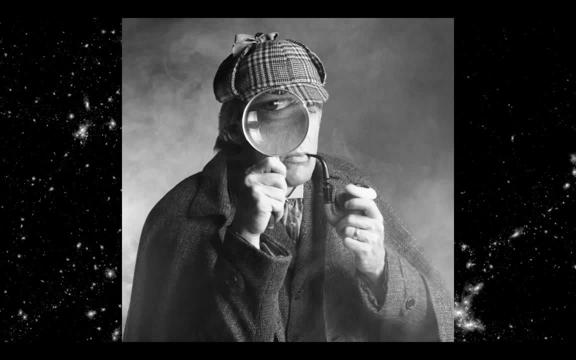 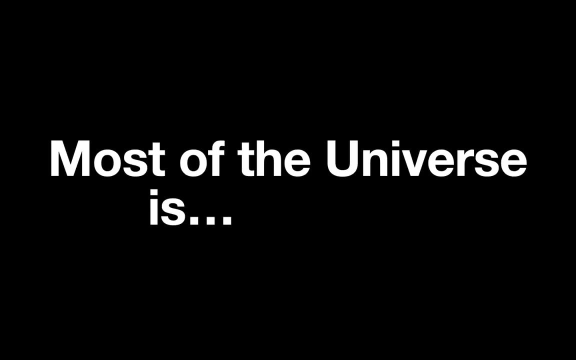 and what I'm going to be talking about today is one of the biggest mysteries of all in astronomy. it's this: most of the universe seems to be missing, so this is the mystery that I'm going to be talking about today. This is the heart of the scientific detective story that I'm going to be introducing. this is 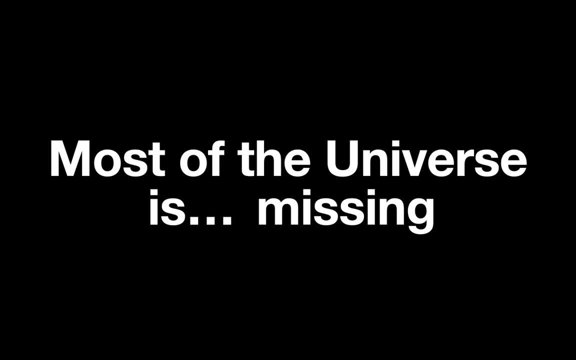 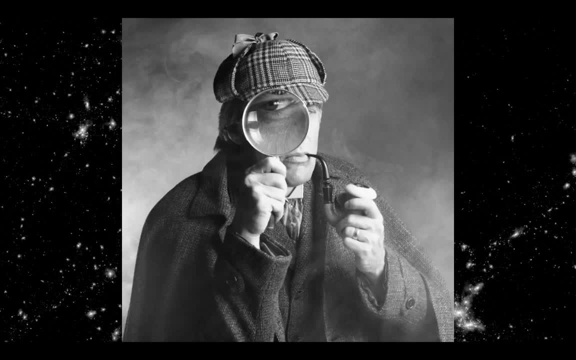 why I love this topic. it's this really really big, exciting question: where is most of the universe? it's the classic detective story, right? something's missing. we have to work out what's going on and, as well as being a detective story, I should also say right up front that this is an unsolved 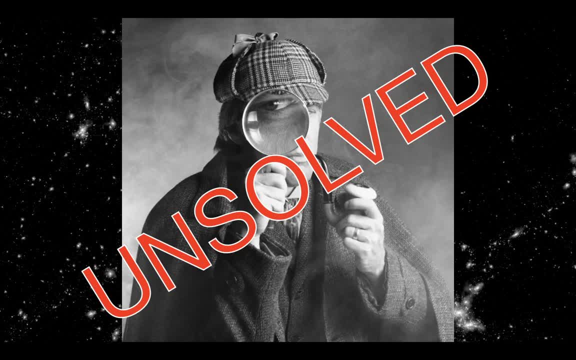 detective story. we know that there is a big problem, that most of the universe seems to be missing. we are doing our best to try and work out what's going on, but right now we're not. now we don't really know the full answer. so, yeah, spoiler for the end, I'm not going to be telling. 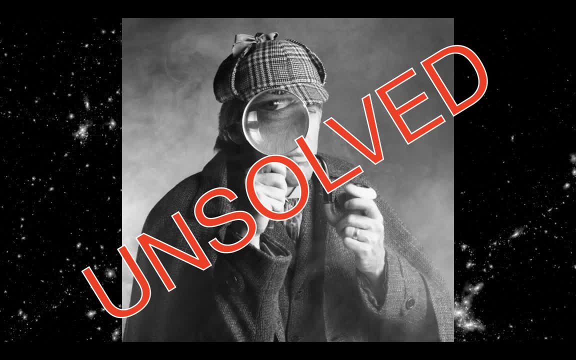 the answer, because we don't know the answer yet. so this can also be a kind of a cry for help for young people that want to grow up and become astronomers. maybe you guys can grow up and become scientists and help us solve these problems. it's going to be a talk in two halves. originally it 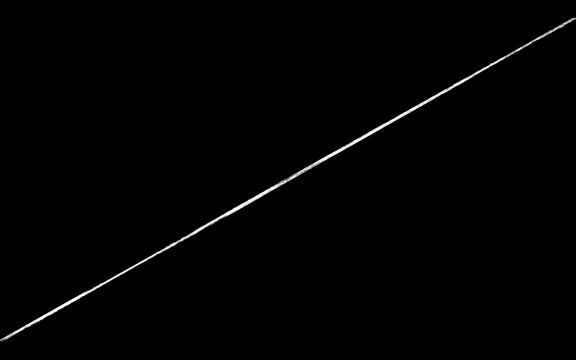 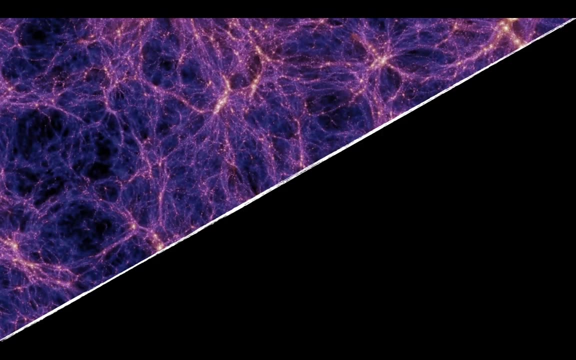 was going to be two halves today, but it's quite a lot of stuff, so we're going to do half this week and half next week, because there's two different types of missing stuff. there's a bunch of missing stuff that seems to glue the universe together, and there's a bunch of missing stuff that seems 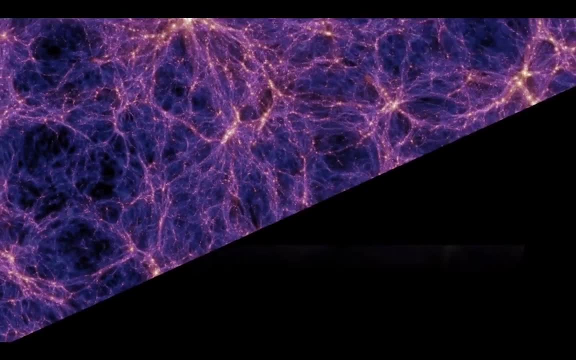 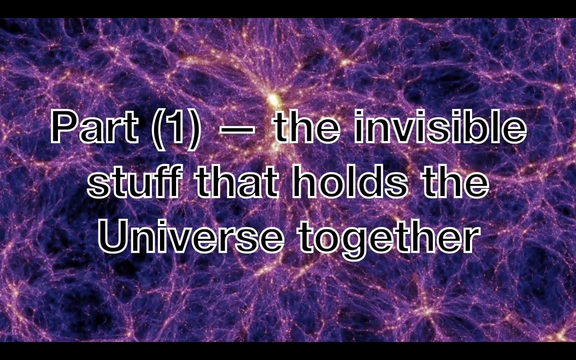 to be doing the opposite, blowing the universe apart. so that second one we're going to handle next week. today we're going to be talking about all this strange invisible stuff that seems to be holding the universe together, and it's going to be the detective story of how we are going about. 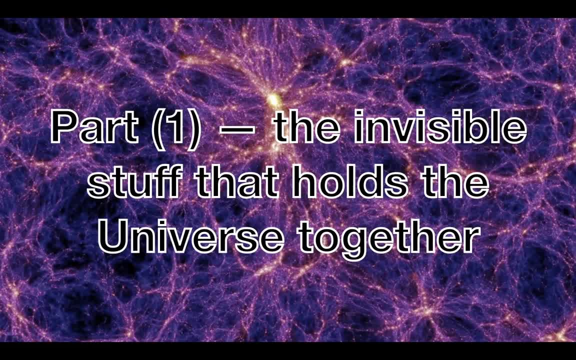 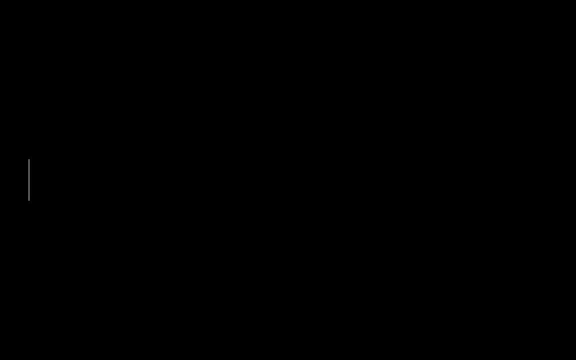 trying to find this stuff, okay. so let's forget universes for a second, because it gets very complicated or it gets quite abstract quite quickly, and let's think of a much simpler question: how do you weigh yourself? if you wanted to find out how much that you weigh right now, what would you do? um, i'm guessing you probably have some scales in. 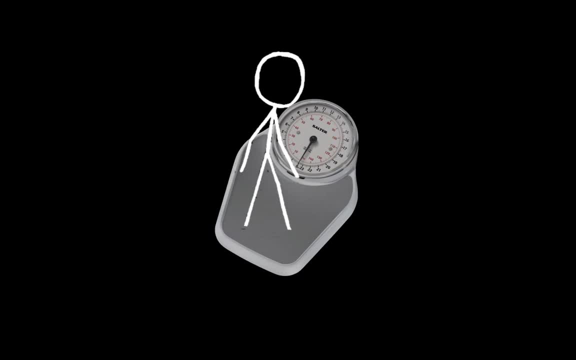 your house, and so you would go and dig the scales out and then you would stand on those scales, right, and then whatever number shows on the scales is how much you weigh. okay, pretty simple, right, but think about what's actually happening, like: why does that? why do the scales give you a number? 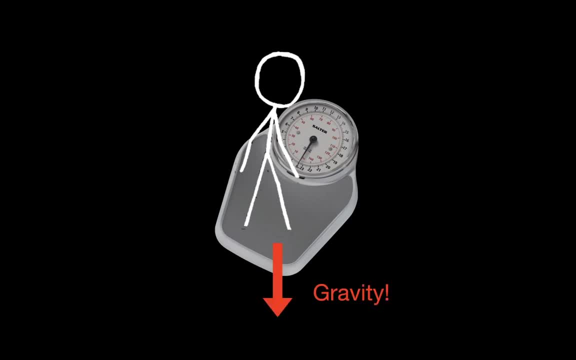 and it's because you're being pulled down by gravity, right? so when you stand on the scales, gravity pulls you down, and then the number that shows on the scales is how much gravity is pulling you down. right, it's a number that represents how strongly gravity is pulling you down towards the. 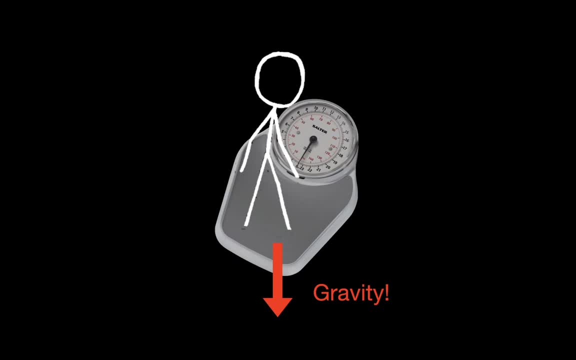 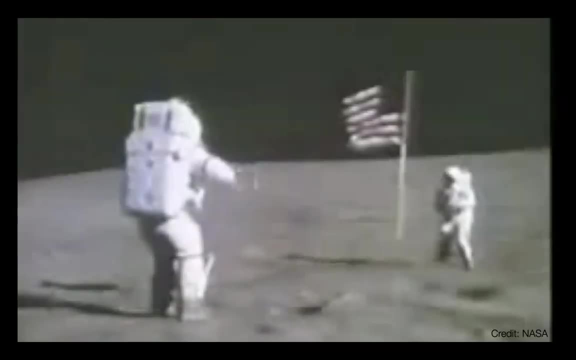 earth, right? so gravity is something that we use when we want to weigh things, and that's what i'm going to be talking about for a bit. how, like that, gravity can be a really useful tool for weighing things? what about if we go other places in the universe? so think about the moon, right? so this? 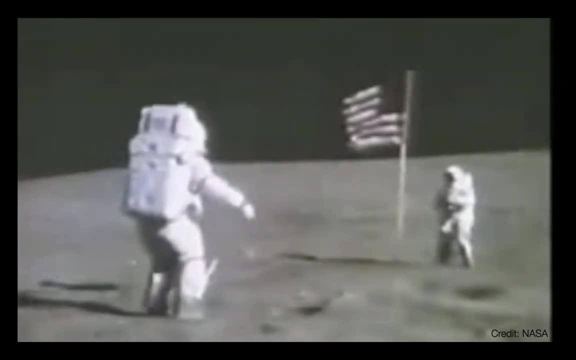 is this nice video that nasa released of astronauts jumping around on the moon, and you can see that everything looks a bit floaty, doesn't it? when the astronaut jumps up in the air, they take a bit of a longer time to go down, so that's a bit of a hint. 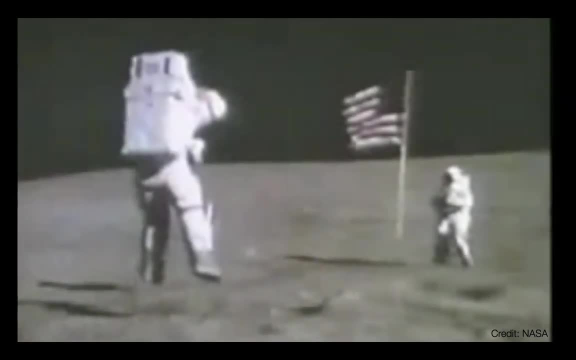 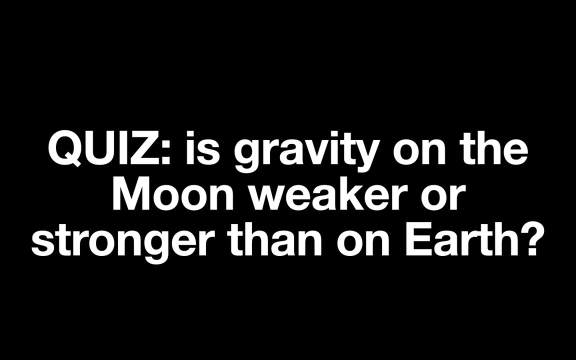 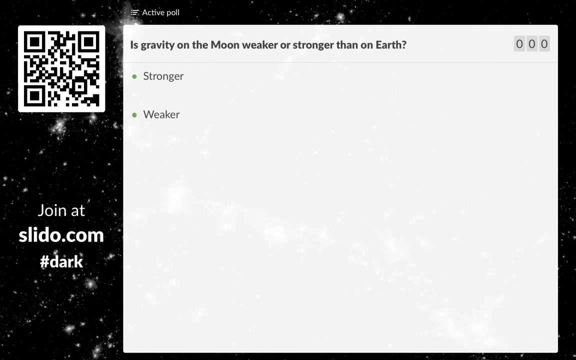 that gravity is behaving differently, and so we're going to come to, uh, the first of today's quiz questions. uh, which hopefully is quite an easy one to start you off. is gravity on the moon stronger or weaker than the gravity on earth? so the gravity on the moon is definitely different to earth. is 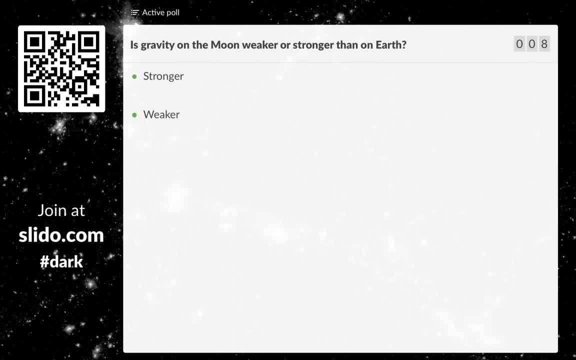 the. is the moon stronger or weaker than the gravity on earth? so the gravity on the moon is definitely different to earth. is the moon's gravity weaker or stronger than the earth's gravity? hopefully this will be a nice and easy one, uh, to get you started. so i'm going to give you a little moment to have a. 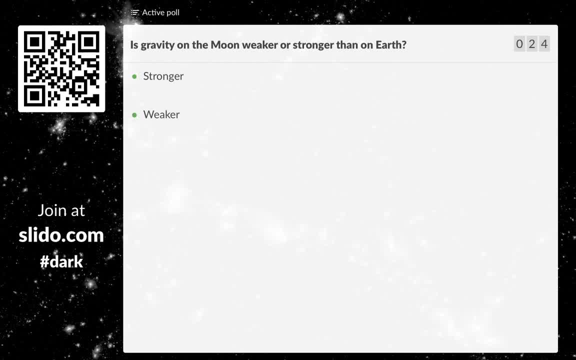 think about that. i can see all lots of fantastic coming uh questions coming through already, by the way. so, yeah, keep keep these coming. um, i might not be able to get to them all because there are absolutely loads of them coming through, but i will do my best to answer many of these, really, really. 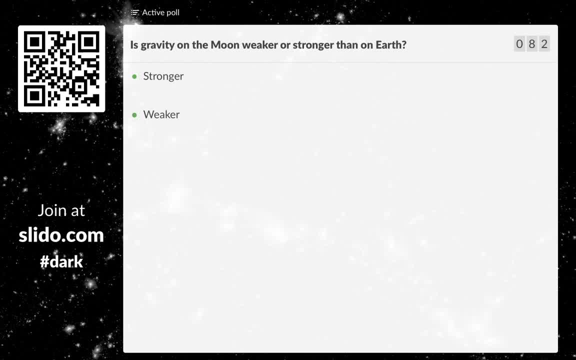 fantastic questions as i can, so i hope you enjoyed this video and i'll see you in the next one. bye, bye, uh, at the end of the talk. okay, is the gravity of the moon stronger or weaker than on the earth? let's see what you're saying. 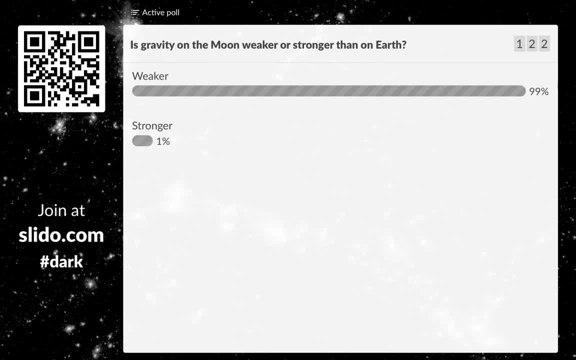 uh, very nice. 99 of you- almost everyone- has got exactly the right answer: the gravity on the moon is weaker than the gravity on the earth. very, very nice. well done you guys. and so the gravity on the on the moon is weaker than the earth. if you could take your scales to 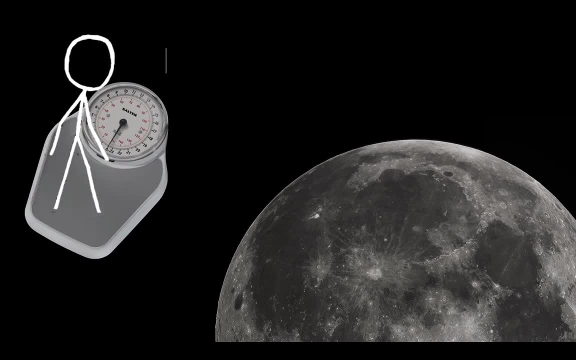 the earth and stand up. sorry, if you take your scales to the moon and stand on them, you would find that the gravity on the surface of the moon is about one-sixth of the gravity on the earth. so you would you weigh six times more on the earth. so that's a nice way to lose weight easily, right? 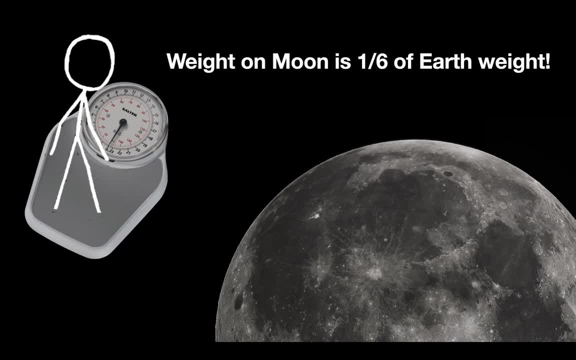 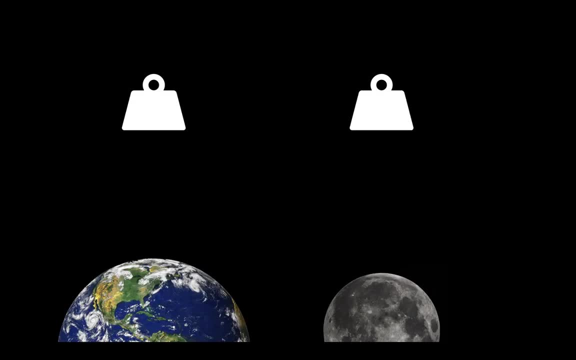 if you could stand, uh, on the moon, uh, and you would weigh 10 kilograms, if you weigh 60 kilograms on earth. and so because the moon's gravity is less, because the moon has weaker gravity on the earth, things like fall more slowly as well, for example, if you imagine dropping a couple of weights. 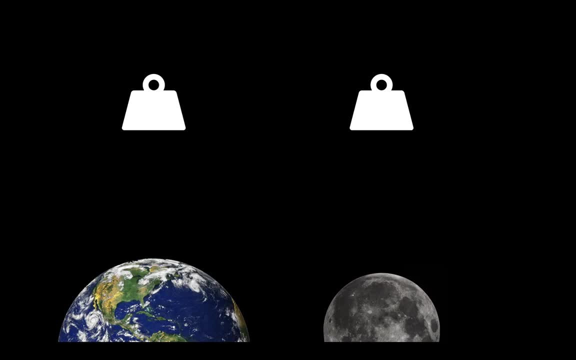 dropping a weight on earth and dropping a weight on the moon. if you drop them at the same time, like now, the weight on the earth is going to fall much faster. right, because gravity is pulling it down harder, and so the point i'm trying to make is that, because the moon's gravity is weaker, we 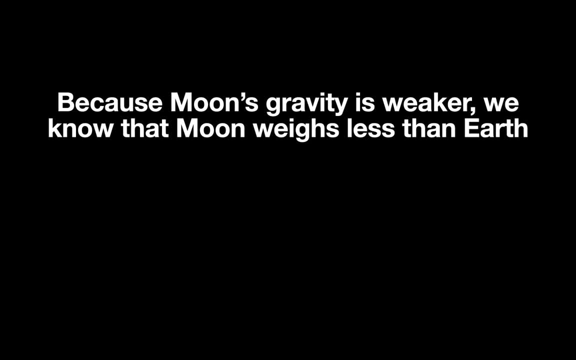 know that the moon has to weigh less than the earth. right, think about what causes gravity. like gravity comes from the fact that the moon weighs something, and so, in general, the gravity on the earth is going to weigh less than the earth, and so, in general, if we want to know how heavy something, 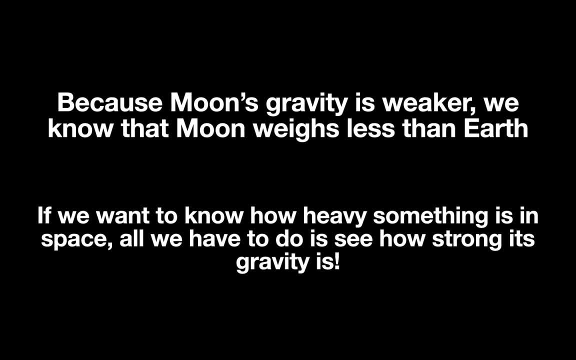 is in space, what we have to do is see how strong its gravity is. this is what i was talking about when i was saying gravity can be a tool to weigh things. if we want to weigh something in space, what we do is we see how strong its gravity is, and that lets us weigh things in space. so what else can we? 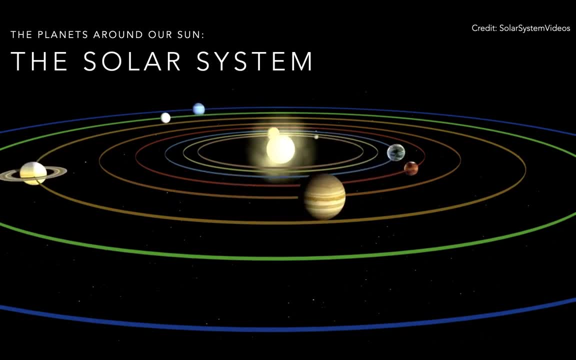 weigh in space. let's find some other things. what about the sun? right? so the sun is the star in the center of our solar system. so the sun is the star in the center of our solar system, right? so this is what we showed uh way back in week. one of these talks comes from this fantastic 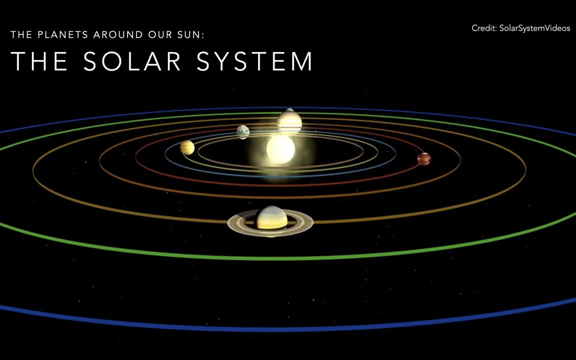 youtube channel solar system videos and it shows this nice cartoon of the planets in our solar system orbiting the sun. so remember the colored lines aren't there right? they're just showing you how the planets are pulled around by the gravity of the sun, and the gravity of the sun is the 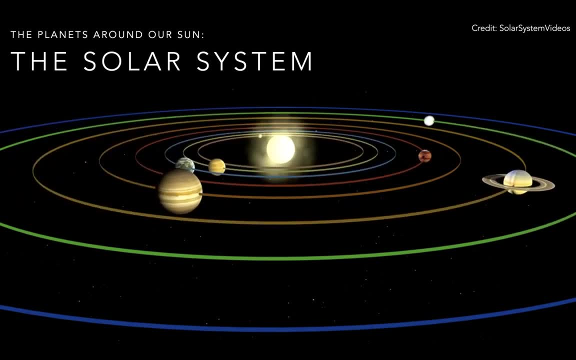 important thing, right. if it wasn't for the gravity of the sun, all the planets would just fly off into the darkness of space. it's the gravity of the sun that holds the solar system together. gravity to work out how heavy the sun is. And the answer is yes, right, We can't put the sun on a. 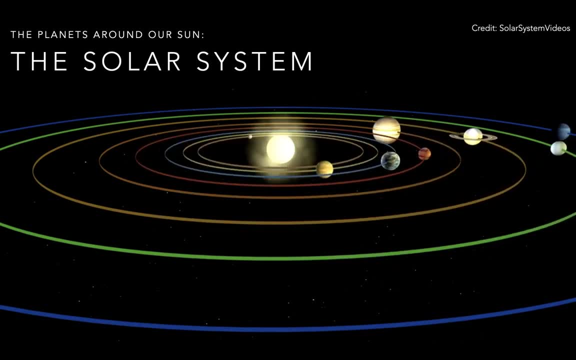 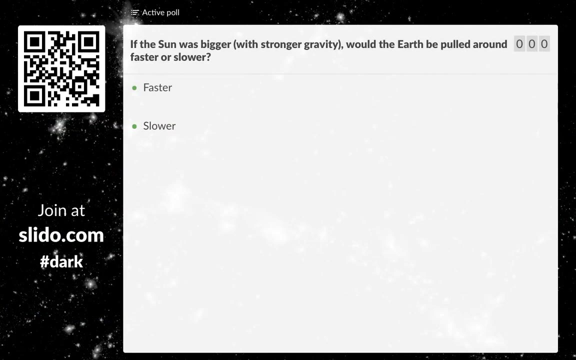 giant pair of some giant cosmic scales to weigh it. But what we can do, we can use the same gravity trick and look at how strong the gravity is and use that to weigh the sun. Okay, so time for the second quiz. This one is a little bit more tricky. If the sun was bigger, like had stronger gravity. would the earth be pulled around the sun faster, or do you think it would go slower? So this can't happen in real life, right? So we're kind of pretending that we have magic powers, So you have a magic astronomy wand and you could make the sun bigger and give it stronger gravity, Do you think? 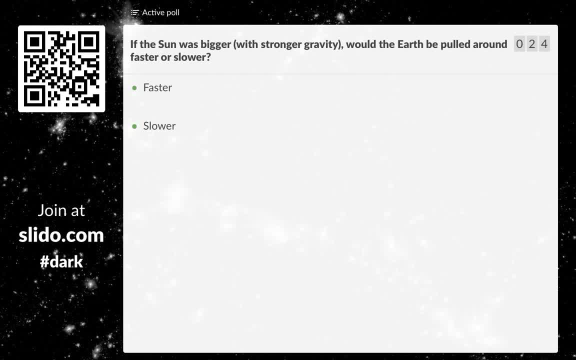 we would speed up or do you think we would slow down? Kind of cool space fact to you. while we're waiting, the earth goes around the sun at more than 60,000 miles an hour, which is the most incredible fact to me. So it doesn't feel like it's going to slow down, but it does. So we're. 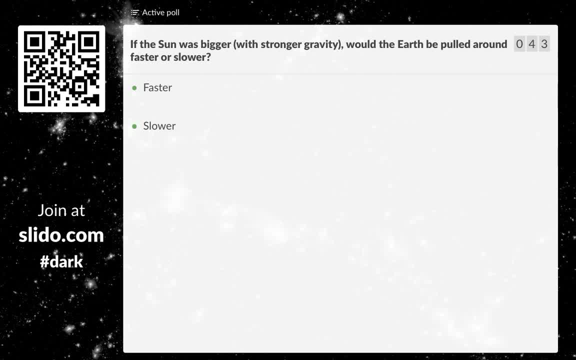 if you shut your eyes right now- I guess, after you voted, shut your eyes and you can know that you're traveling right now at more than 60,000 miles an hour around the sun. It's amazing that we could be traveling so fast without realizing it. Okay, let's see what you guys are saying to. 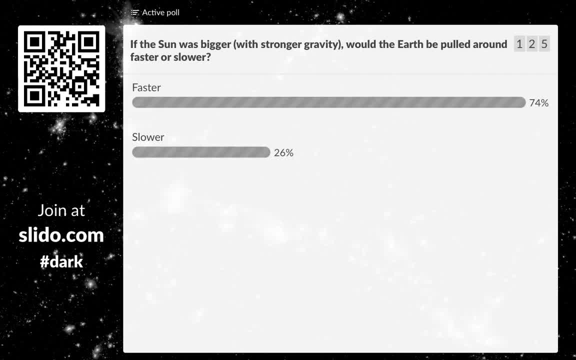 this one. This one is a bit more tricky, But, yes, three quarters of you have got exactly the right answer, Well done. If the sun was bigger, would the earth be pulled around the sun faster? If the earth was bigger has stronger gravity than the earth, would be pulled around faster. 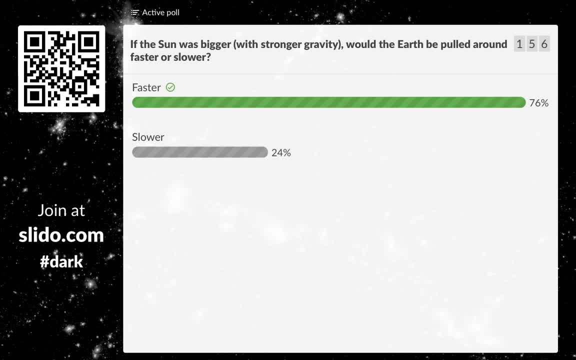 which kind of it makes sense if you think about it right, If you think of gravity like, like, being the strength of something. if you're stronger you can move things around easier and move things around faster. So with stronger gravity, earth would be pulled around the sun. 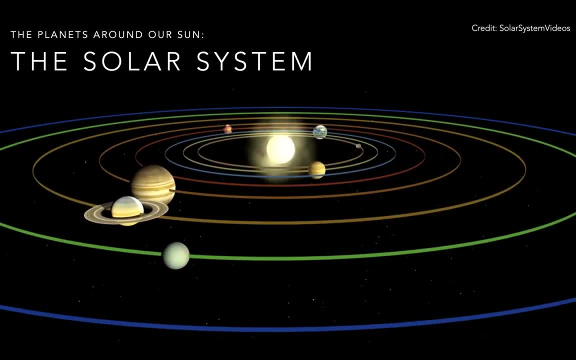 much faster than we are at the moment. So yeah, we're going at this: 60,000 miles an hour or something a bit more than that. If we can make the earth bigger, oh sorry. if we can make the sun bigger, we would speed up. If we would. if we can make the sun bigger, we would speed up. 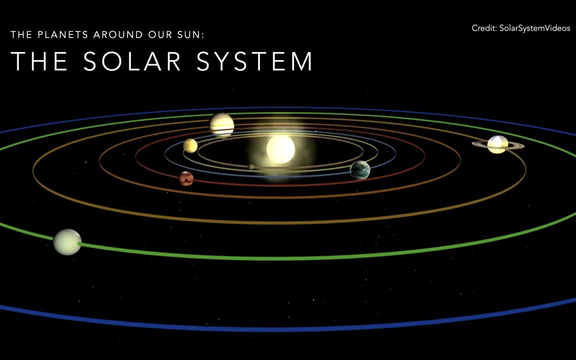 If we can make the sun smaller, we would slow down, But the speed we're going gives us the weight of the sun And that turns out that is about a million times heavier than the earth And we know that because of its gravity. right, We didn't get some giant cosmic scales and put 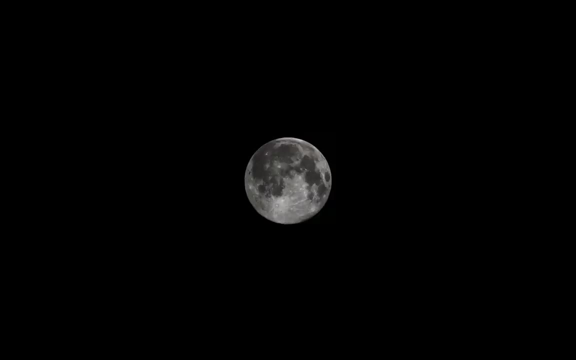 the sun on it. We just measure the strength of its gravity And luckily this works for everything in space. So whenever you find out that astronomers have weighed something in space and we say this is how much something weighs, this is how we work it out: We just look at the gravity. 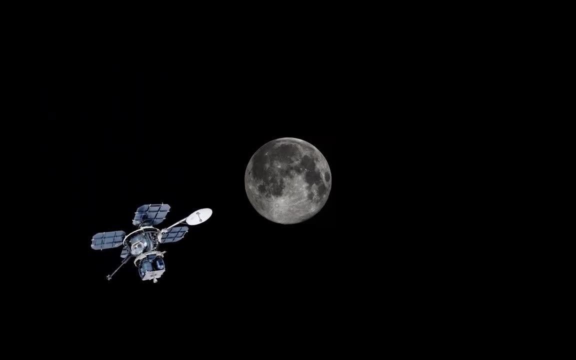 So we can weigh the moon, for example, by get by taking a spaceship that's going around the moon and we just look at a spaceship orbiting the moon And, depending on how fast that spaceship is going, we can use what we know about gravity to weigh the moon. So that's how we know that the 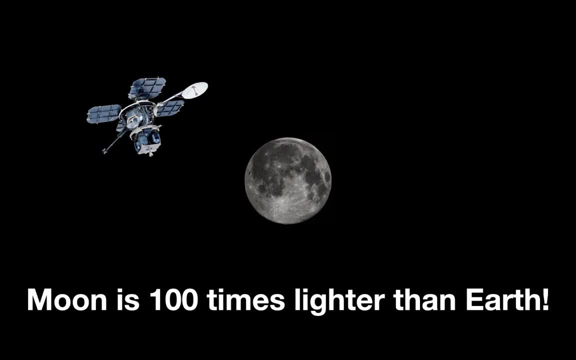 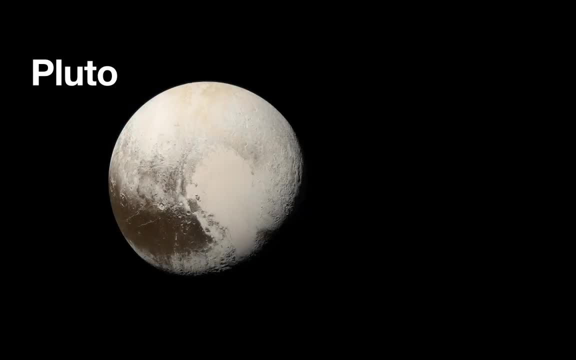 moon is about a hundred times lighter than the earth, right, The earth is a hundred times heavier than the moon. We know that because of measuring the gravity of these things. Pluto is another cool one, right? So Pluto, when it was first discovered, we didn't really know how much it. 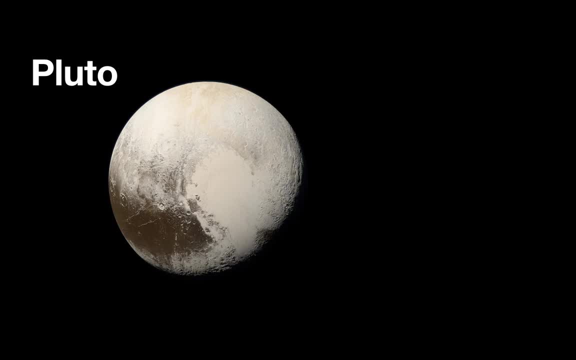 weighed. It was a bit of a mystery. It was just this teeny tiny dot on the edge of the solar system. How do you weigh a teeny tiny dot on the edge of the solar system And we just look at the dots. We kind of can't right. But we were able to weigh Pluto when we found out that Pluto has a 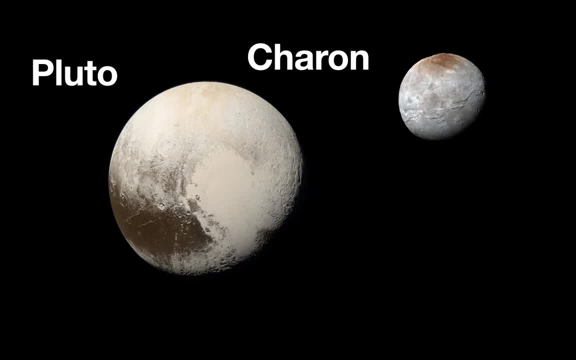 moon called Charon, And we can watch this moon going around Pluto, measure the gravity of Pluto and then that tells us how much Pluto weighs, which is about five times lighter than the moon. So this trick is amazing: We can just weigh something that's like billions of miles away. 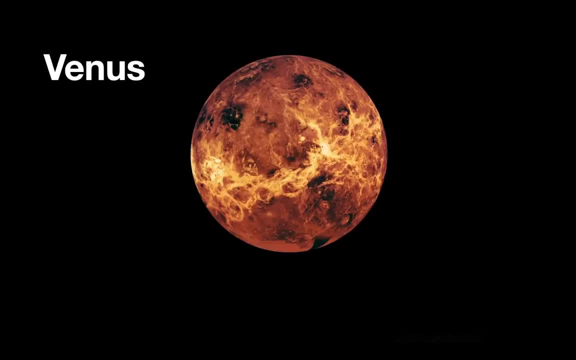 in the solar system, Venus is a really, really interesting one. So Venus doesn't have any moons, So you'd think it would be quite difficult to work out how heavy Venus is. But it doesn't always have to be a moon. You can just look for things like asteroids and 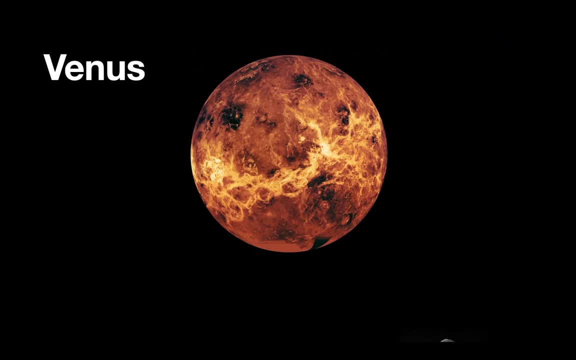 meteorites. So when little meteorites go past Venus, we can watch them being tugged around by Venus's gravity. Then that tells us how strong the gravity is on Venus, which tells us how much Venus weighs, And so we know that Venus weighs about the same as the Earth. So this is great. 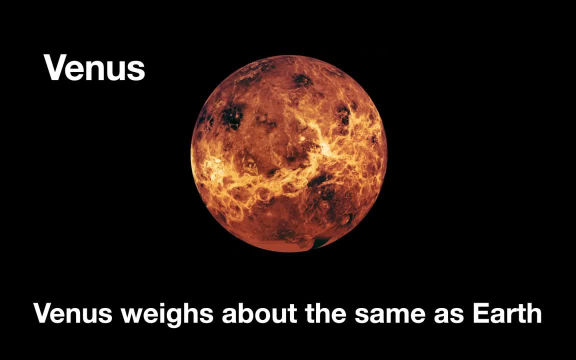 We have a trick that we can just look at the gravity of something and it lets us weigh things. And so we can weigh stars, we can weigh planets, we can weigh all kinds of things in space. What about bigger things? Do you think we can go bigger and weigh something else? 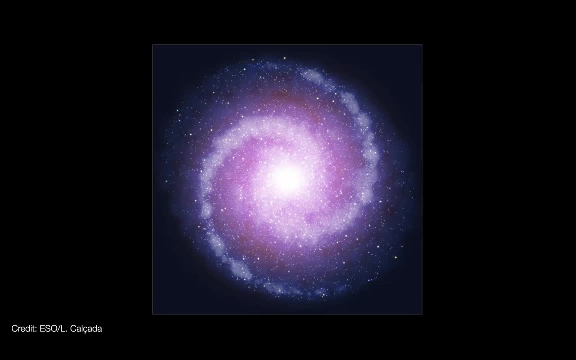 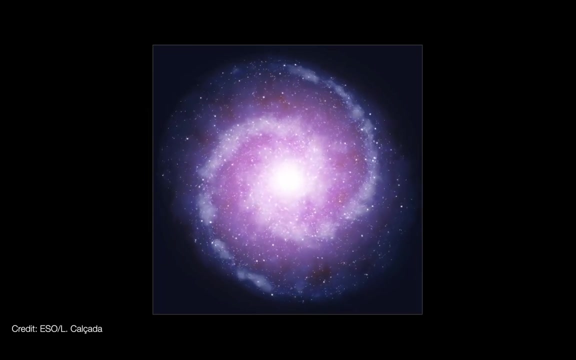 So what about a galaxy? So galaxies are really cool things. Again, I spoke about these in week one. We're part of the Milky Way galaxy. The Sun is just one of about 200,000 million stars in our Milky Way And galaxies, just like the solar system, kind of rotates, with all the planets going around the Sun. 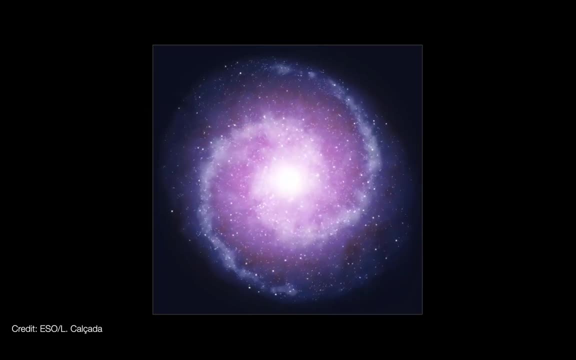 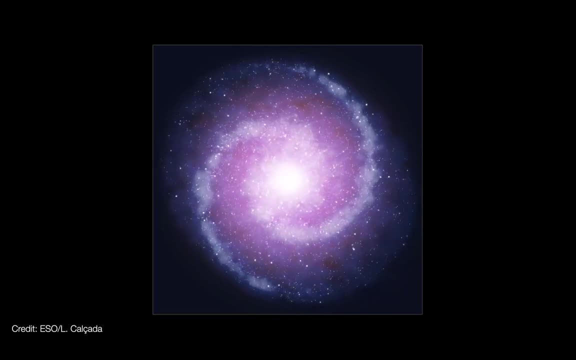 And so the Sun is being pulled around by the gravity of the Sun. They take a long time to go around, so the Earth does a lap of the Sun in a year. The Sun does a lap of the middle of the Milky Way in about 220 million years. So it takes a lot, lot longer to go around, But even still we should be. 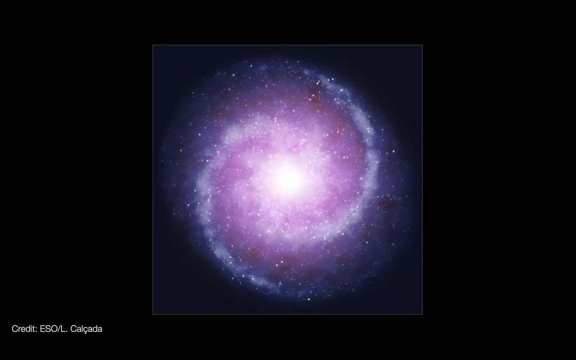 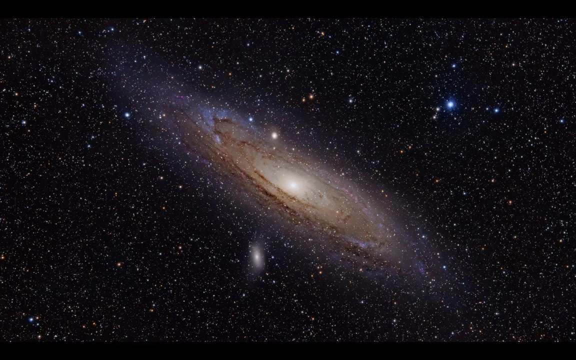 able to use our trick right, We should be able to look at stars in a galaxy, measure how fast they're being pulled around, and that lets us weigh a galaxy, which is an amazing thing if you think about it. This giant thing, you know millions and millions and millions of stars are being pulled. 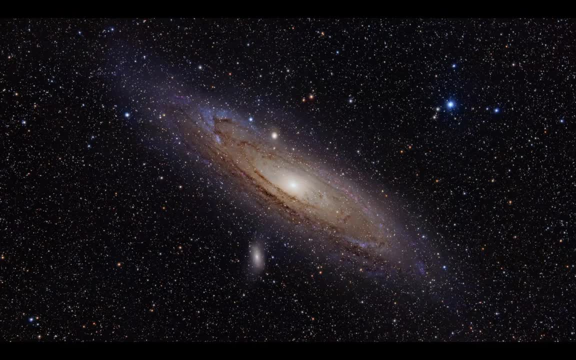 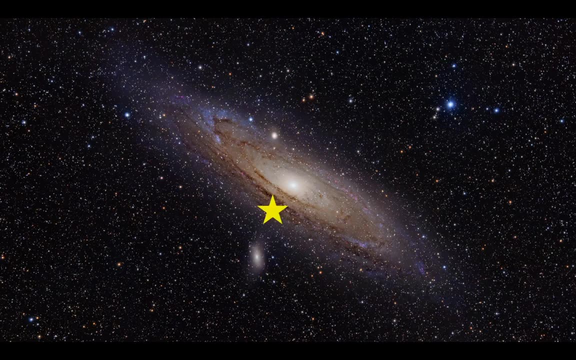 around. millions and millions of stars are being pulled around. millions and millions of stars are being pulled around, containing hundreds of thousands of millions of stars. We can just work out how much it weighs, So we do the trick. So this is the Andromeda Galaxy. That's the nearest big galaxy to our Milky Way. 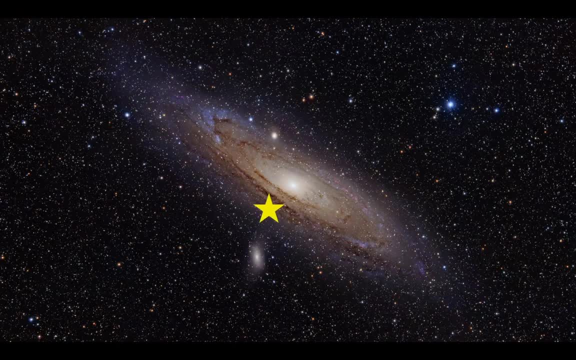 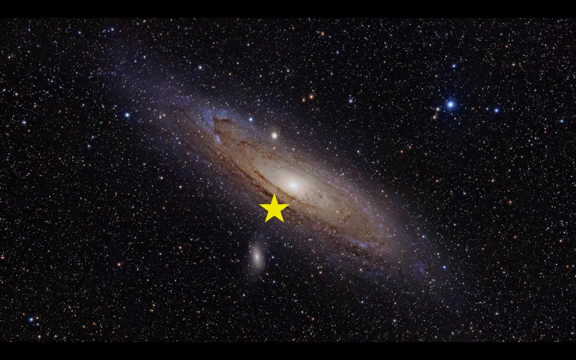 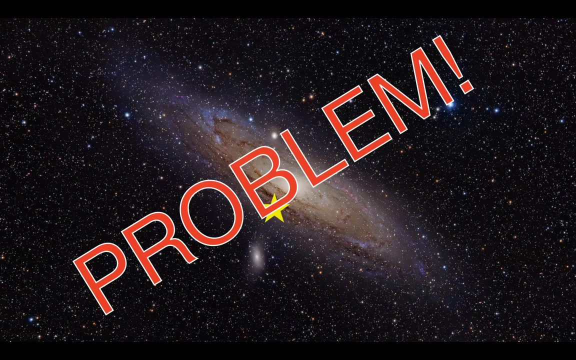 We can just look at a bunch of stars, look at how fast these stars are being pulled around, and that lets us weigh the galaxy. We can use our gravity trick again. Easy, right, Well, no, Unfortunately, at this point we hit a very, very interesting problem, And this is where today's topic comes in. 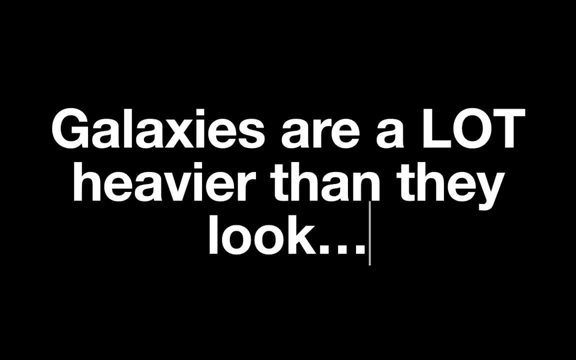 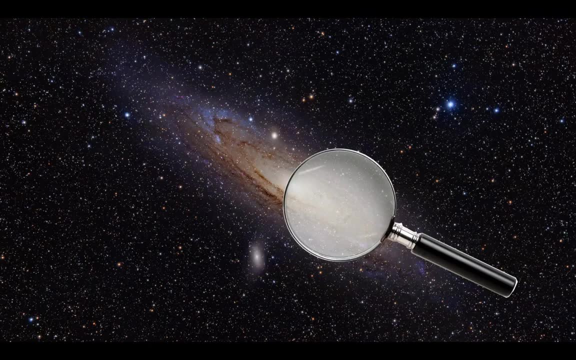 The problem is this: Galaxies are a lot heavier than they look, And by a lot, I mean like a lot, lot heavier than they look. So what does this mean? What does it mean to say that a galaxy is heavier than they look? Well, you can take a look at this galaxy right, Or take a look with a telescope and 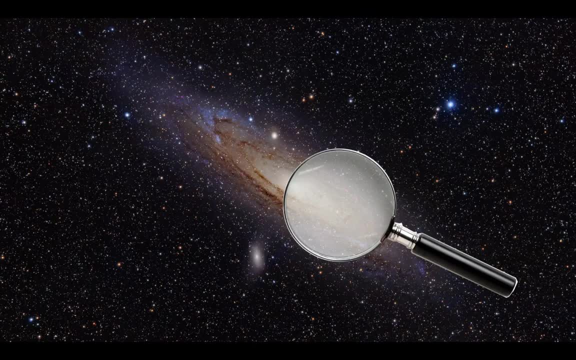 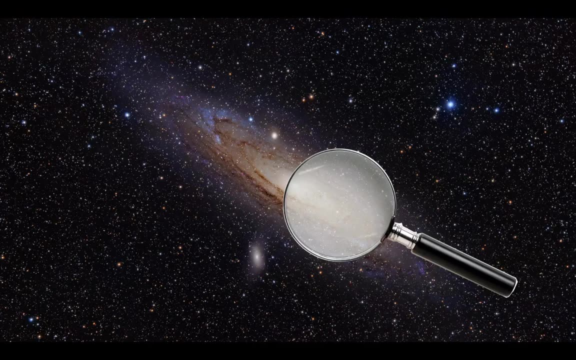 look really carefully and you can get a rough idea of how many stars are in our galaxy, right? Like I said, our Milky Way has 200,000 million stars inside it, So you can look at a galaxy and get a rough idea of how many stars are inside it, which could give you a rough idea of how much it weighs, right? 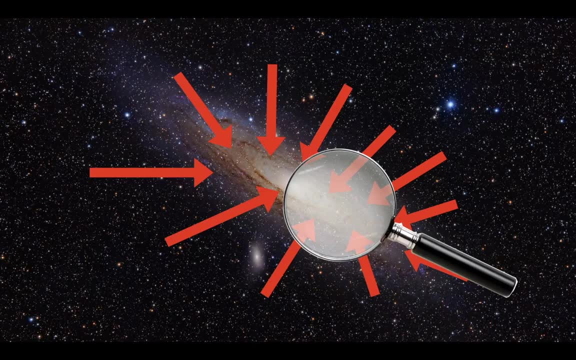 Galaxies are big clouds of stars. You count the stars and you've pretty much got a rough idea of how much the galaxy weighs, But it turns out that's just completely wrong. When we use our clever gravity trick, it turns out that galaxies are way. 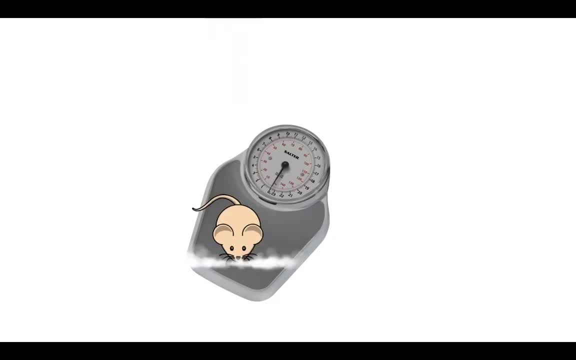 way, way heavier than they should be, which is really really odd. It's kind of like you're weighing something very light, like you're putting a mouse on a pair of scales and then your scales tell you that you're weighing something. 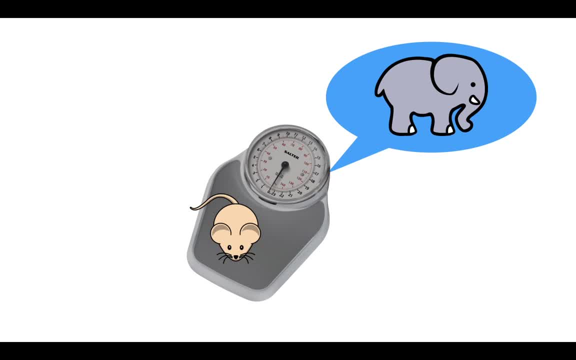 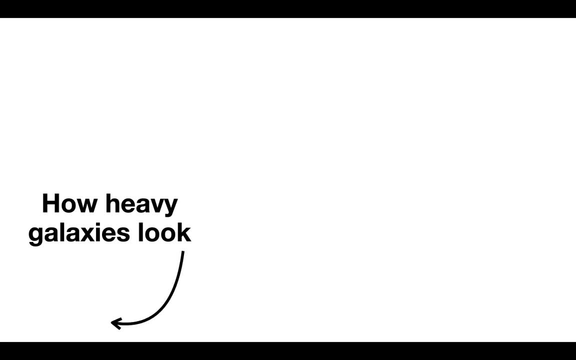 very heavy indeed. That's weird. That tells you that there's something wrong here or there's something very strange going on that we don't expect. So galaxies are about 10 times heavier than they look, which is a huge amount, right? So if this is how heavy galaxies look, this is like 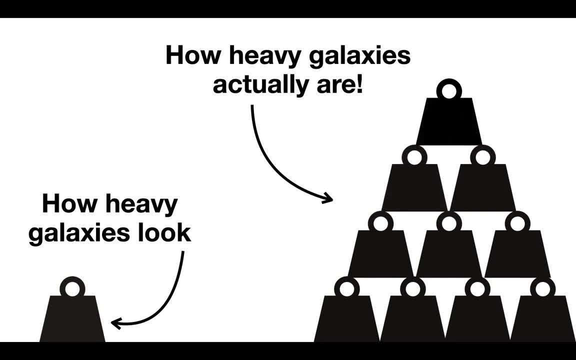 a representation of how heavy galaxies actually are. So like 10% of a galaxy's weight is absolutely fine. That's the stuff we can see. That makes sense. But most of a galaxy seems to be this weird invisible stuff that we can't see, And so we can't see it, And so we can't see it, And so we can't. 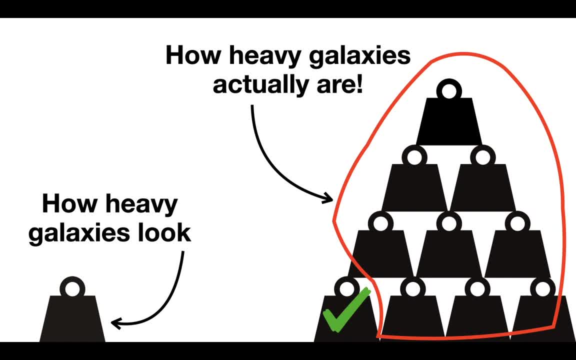 see that stuff That we know it's there because we can see it's gravity, we know it weighs something, but we just can't see it at all. So what is this stuff? Why are galaxies full of this weird invisible stuff that seems to weigh something but we just can't see it? And this actually. 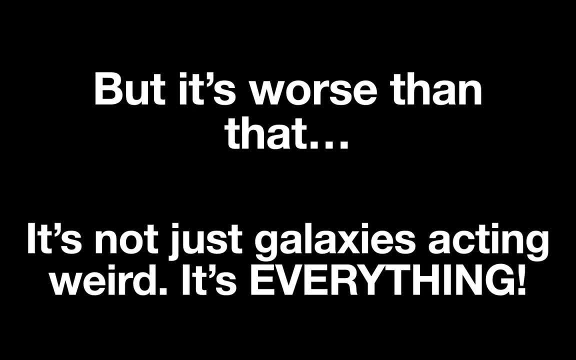 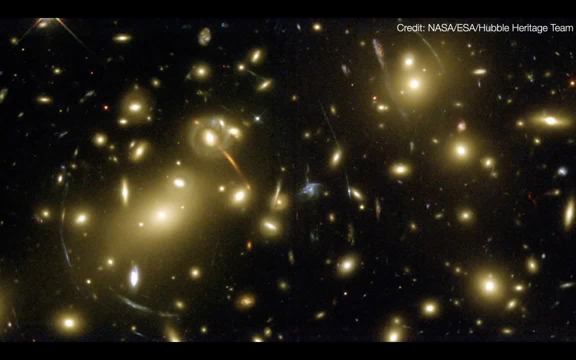 gets worse than that. so I've been talking about different things in space and I've said that galaxies act weirdly. It's not just galaxies that act weird, it's actually everything, Whenever we put our telescopes to anything in the universe with anything big – so we 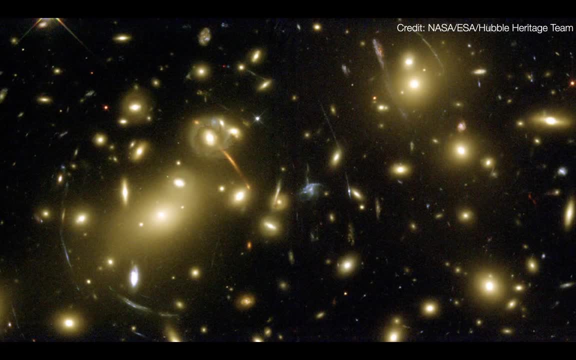 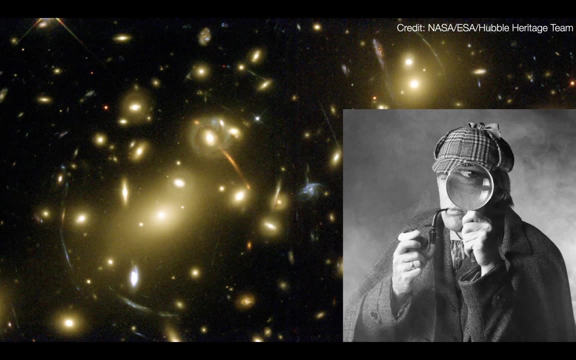 or clusters of galaxies or even the entire universe itself. we see this exact same problem. We see that everything is heavier than it should be. So this weird like invisible stuff that seems to be weighing down galaxies, that seems to be absolutely everywhere, The whole universe. 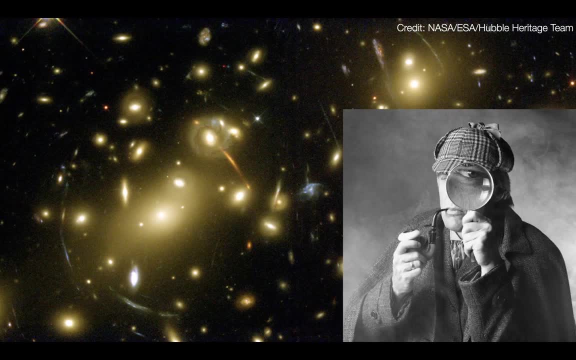 is much, much heavier than it looks. It looks like there's a bunch of invisible stuff in the universe. We know it's there because we can see the gravity of it. we can see that it weighs something, but we can't see it at all. So what's going on? What is this stuff? And the answer is: 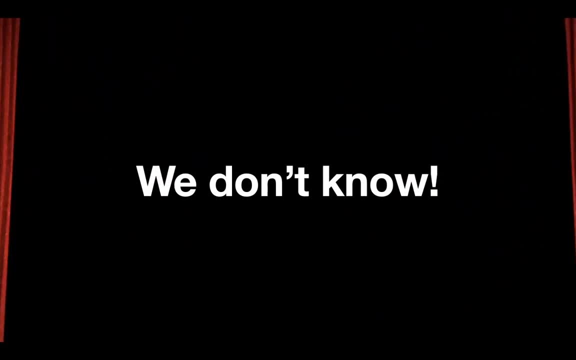 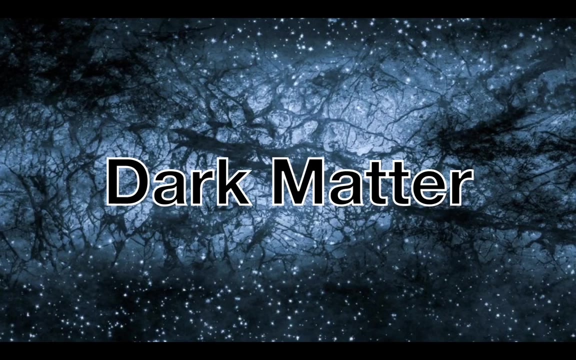 we don't really know. It's a mystery. This is why I call this a scientific detective story. We know this stuff exists. We really don't know what it is. So what we call it is dark matter, right, So matter here means that it's stuff. you know, it's some stuff that's out. 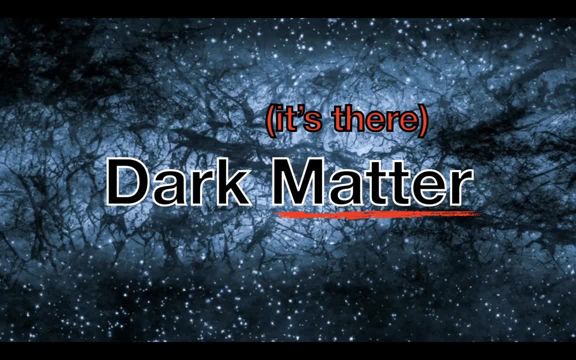 so matter is just a scientific word meaning stuff. right, Like I'm made of matter, you are made of matter. your house is made of matter. Matter just means stuff. So dark matter is stuff that's there, but it's invisible. That's why we say it's dark. So dark matter is invisible stuff. 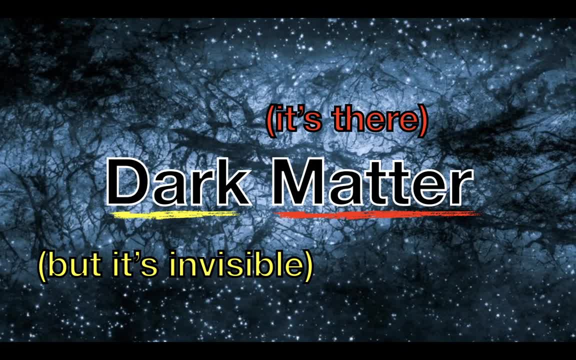 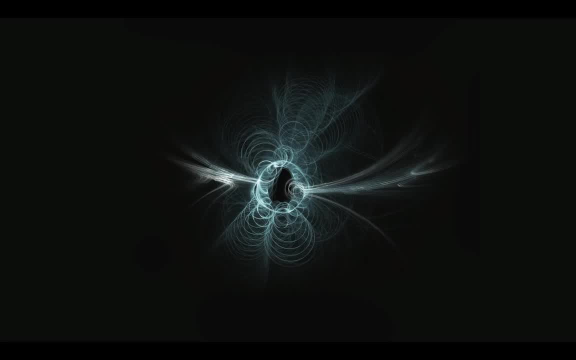 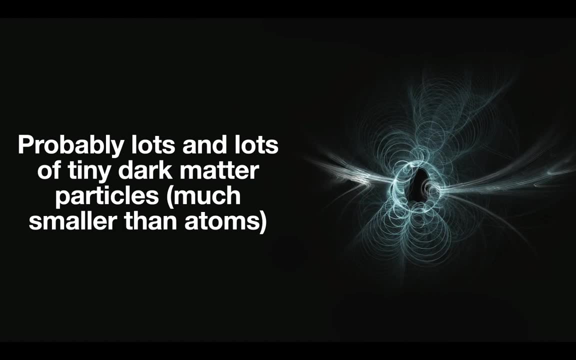 We know it's there because we can weigh it. we can't see it, So we know we live in a universe full of dark matter And our best guess- so this is a kind of a nice drawing of just some kind of our best guess- is that dark matter is some kind of teeny, tiny particle so much, much smaller than 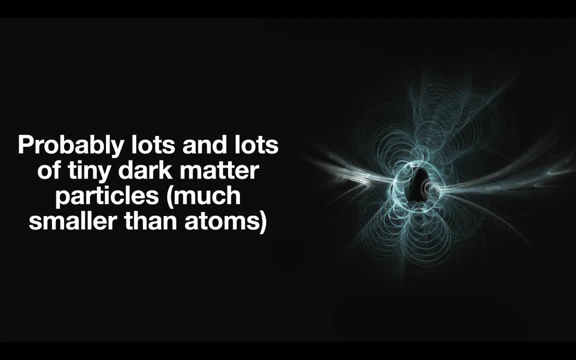 an atom, right? So our best guess is that the universe is full of just an absolutely ridiculous number of these tiny, tiny particles, like a whole sea of these tiny particles that is just filling the universe, And that's our best guess at what dark matter is. We don't really know what. 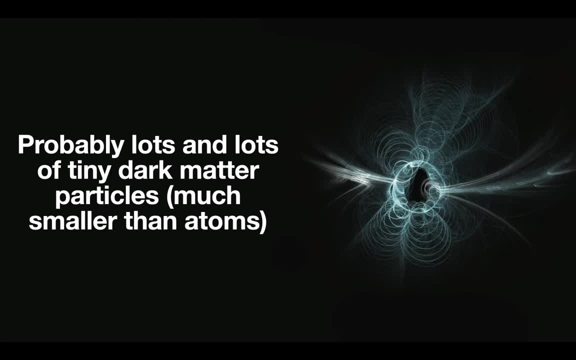 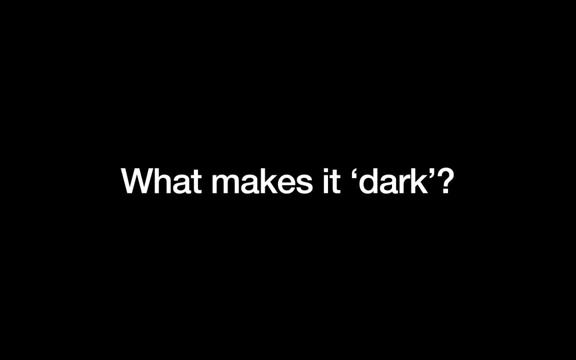 these particles are or how they work or anything like that, but that's just our from looking at the universe. that's our best guess for what's going on. Why is dark matter dark Like? if the universe is full of these particles, why can't we see them? 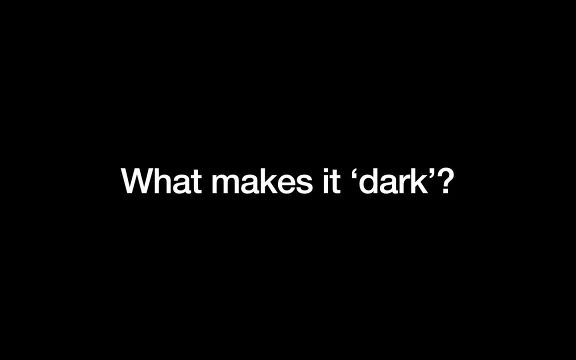 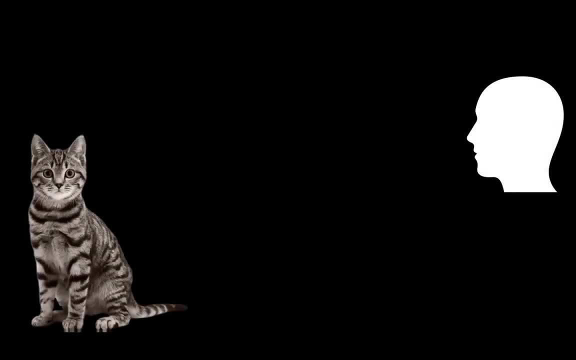 right. If there are so many of them, you think we should just be able to look around and they should be everywhere. Why is dark matter dark? So let's think about how you see anything at all. How does looking at stuff work? So say you want to see an object like a cat or something You need. 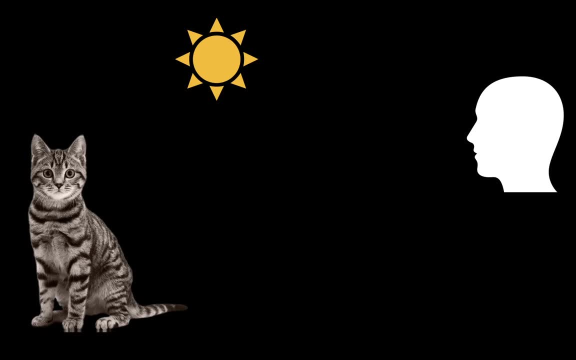 some light to be able to see things. And the way you look at things, the way you see things, is that light comes like reflects off them, right? So light from the sun will come down, hit an object and go into your eyes and then you can see that thing. Or, for example, you're looking at your 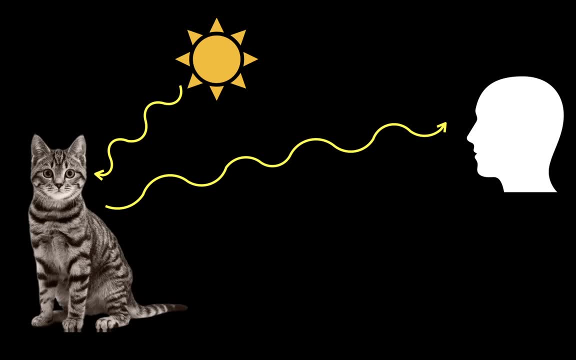 computer screen. now, right. The way you can see this picture I'm showing you is because light is coming out of your computer screen and going into your eyes. Look at the wall next to you, right? The reason you can see that wall is because light is bouncing off the wall and then going into your. 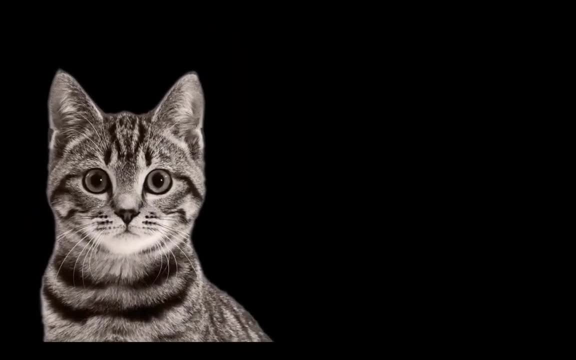 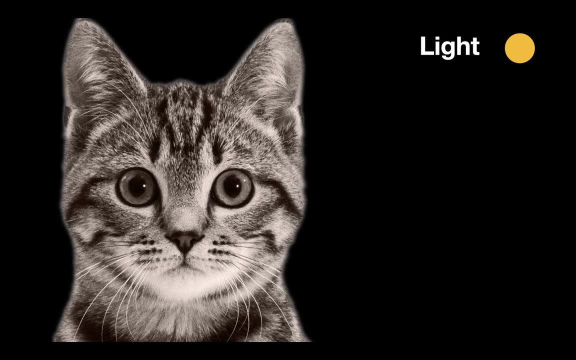 eyes, If you look really closely at what's going on. right, Let's zoom in. So what's happening? You have some object and then you have like bits of light, called like photons or waves of light, and they are crashing into the object and bouncing off right. That's what reflecting is right. 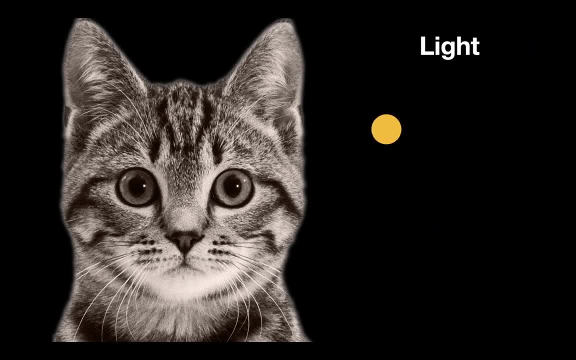 That light hits the object and bounces off, And so that's how you see things right. If light didn't bounce off this object of light, just kind of pass straight through it, then we wouldn't see it. It would be invisible. You need reflection to be able to see things right. You need light to be able to. 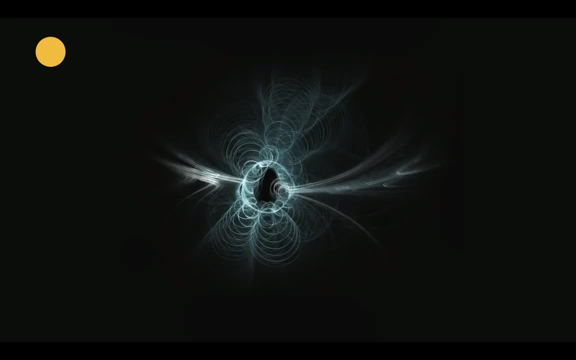 bounce off something, and then that's how we see something. And so this is why we think dark matter is invisible: because light doesn't bounce off it right. So you have a dark matter. some light light will just happily go straight past dark matter as if it's not even there. 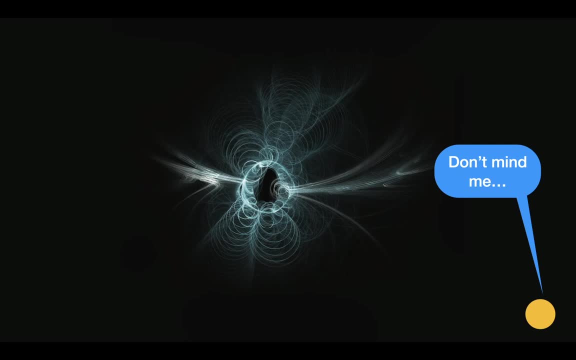 And that's what. that's why this stuff is invisible, So that you know. there can be loads of these dark matter particles out there in space, but any beams of light that go past them just go straight through and out the other side as if they're not there. And so, because dark matter 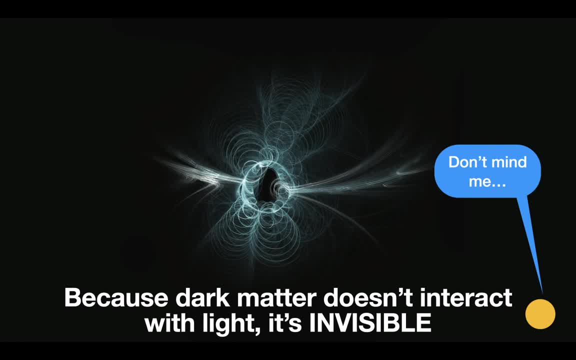 doesn't interact with light at all. that's why it's invisible. That's why this stuff is so hard to see. And by light, of course, I don't- I don't just mean the light we can see, I mean 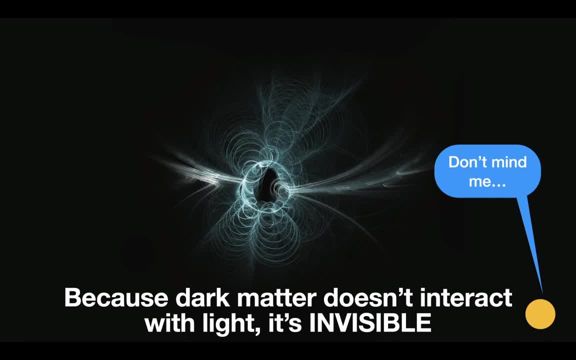 stuff like radio waves or infrared or all of the types of light that we use to study the universe. dark matter ignores all of it, which makes it really, really, really, or it all makes it impossible to see. So dark matter doesn't just ignore light, It ignores pretty much everything. 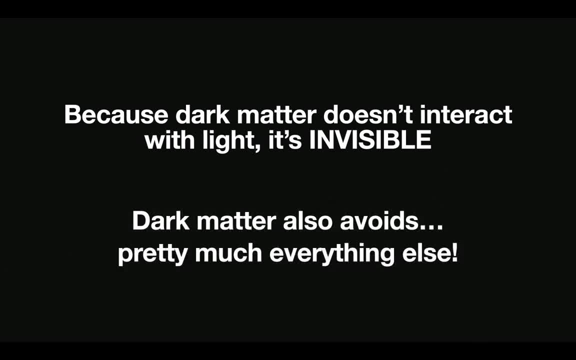 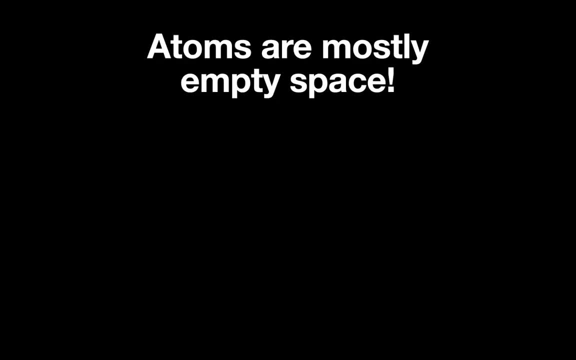 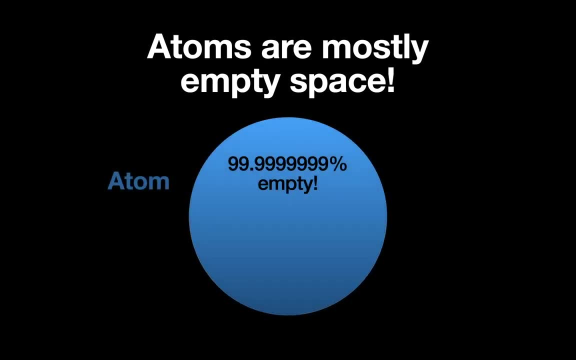 else as well, Like, dark matter is the original social isolator, right? Dark matter avoids pretty much everything else, And one of the things that dark matter ignores are atoms. So remember we were last week about how atoms are mostly empty space, right, So atoms have a nucleus. there's a little. 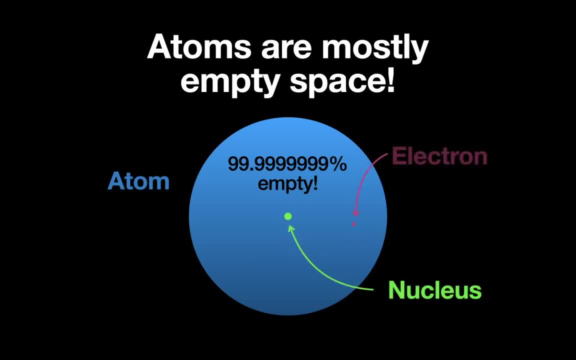 dot in the middle and some electrons. but most of atoms is just empty space, right? 99.9999999% empty space, right. Dark matter can just waltz through that empty space as if the atom isn't there. So because atoms are almost entirely empty space, dark matter just happily passes through. 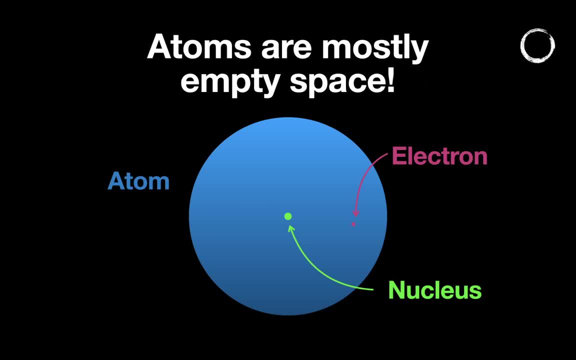 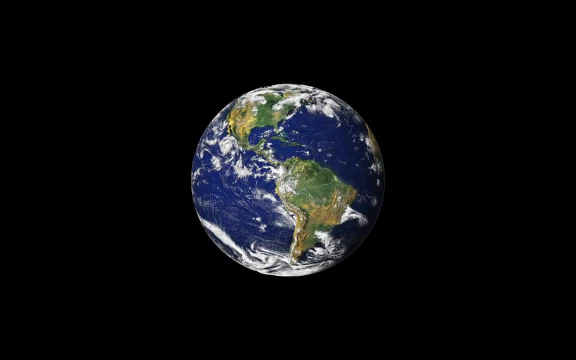 and out the other side, as if atoms aren't there. Dark matter just passes through atoms Really, really easily, Which also means that dark matter can just pass through anything that's made of atoms. So, like the earth is made of atoms, dark matter can just go through the earth and out. 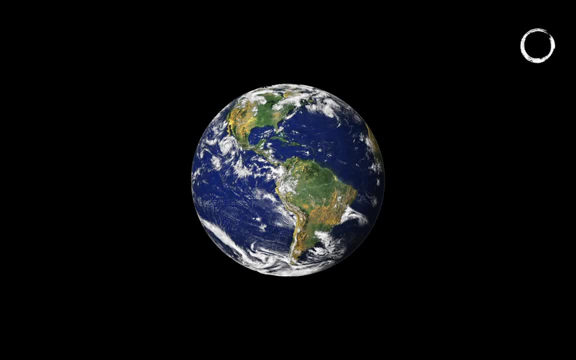 the other side. So this is why it's hard to find right. We can see that space is just full of this dark matter everywhere, but it's just it, just. it's like rain, It just kind of streams through the earth and out the other side, And that's true of anything made of atoms as well, So like 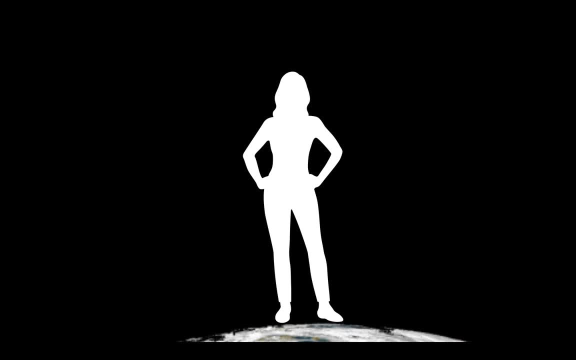 you know, we're made of atoms, My body is made of atoms, Your body is made of atoms, And so dark matter can just go straight through your body and out the other side, as if it's not even there. And so we now think, or we now, you know, we're now almost certain- that there are. 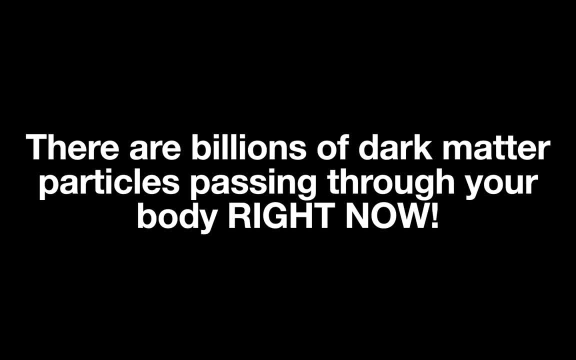 billions of dark matter particles passing through your body right now. There's so much dark matter out there in space. It's just streaming through your body right now. So if you put your hand out and look at your hands like there are billions of dark matter particles passing through your hands. 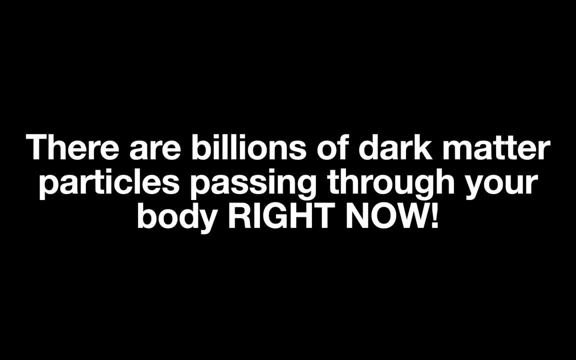 like this very second, But from a dark matters point of view, like you barely exist, right, You're just kind of you. just they just go through your body and out the other side, And so dark matter can just go straight through you and out the other side as if you're not even there. 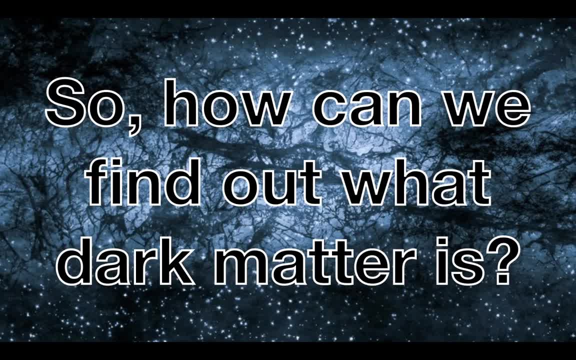 So how can we find out what this stuff actually is? right, We can see this stuff out there in space. We know it's there because we can. you know we can see its gravity. How can we find out what it actually is? What we want to do is build some kind of machine that can detect dark. 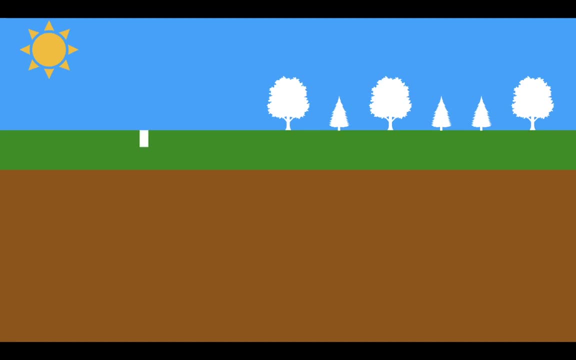 matter. We want to be able to find it so we can learn more about it, And so what we do? we go deep underground, So we dig big tunnels, or, more often than not, we use tunnels that are already there. right, We go down into a big mines. 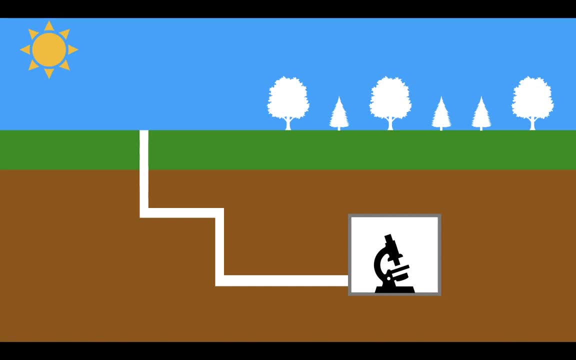 And then deep underground we build machines that can detect dark matter, And then the idea is that if a dark matter particle comes along, it can just pass through the earth as if the earth isn't there, because that's what dark matter does, And then, when it hits our machine, our machine goes. 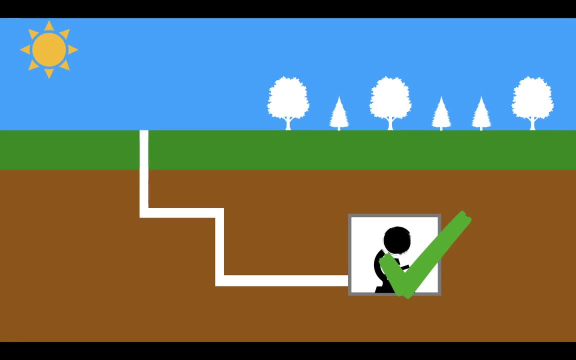 and detects the dark matter, And then we can say, great, we found it. The reason we go underground is because there's all kinds of particles flying around all the time. right, The sun spits out cosmic rays, but most of these particles just can't go through the ground right? 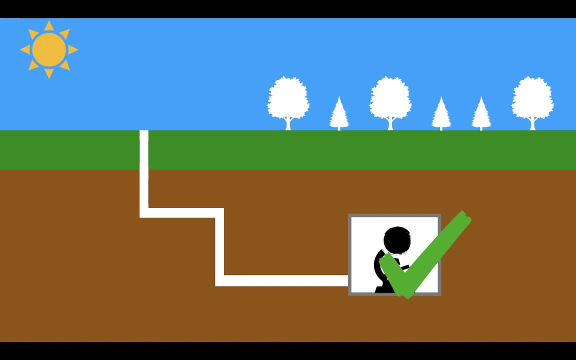 That's something that like pretty much only dark matter can do. So most of the stuff from space just hits the ground and bounces off And then say: if you build your dark matter detecting machine deep underground and you find something, you can be pretty sure it's dark matter, because only dark 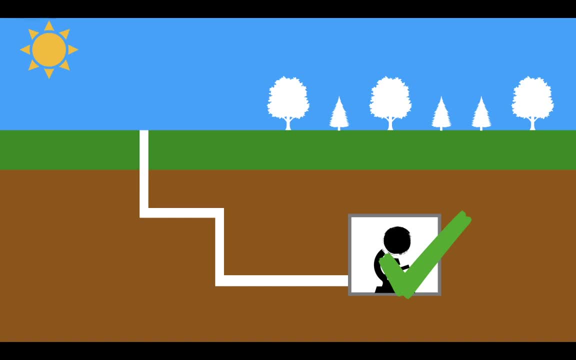 matter can kind of happily waltz through the earth as if it's not there. So this is what we do, right? We go deep underground, We build these dark matter detecting machines to try and catch some of these dark matter particles as they just kind of waltz through the earth. This is a picture. 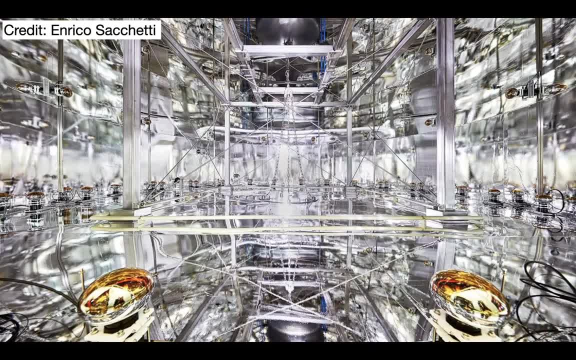 of one of them. They look super cool. This is one of these dark matter detecting machines that's down in Italy. It looks like some super sci-fi spaceship, or doesn't it? So this is one of these things that's deep underground and is trying. 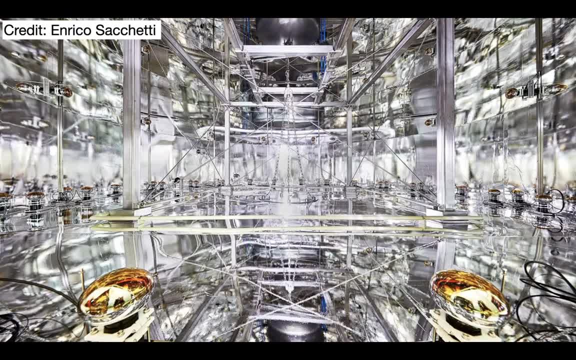 to detect these dark matter particles. There are lots of these all over the world. They all have kind of different designs, but they have one thing in common, which is that so far, none of them have been able to detect dark matter. So far we haven't found any of this stuff, And if you think about it, 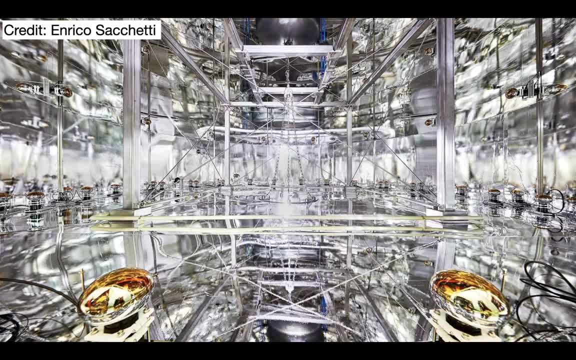 for a second. the reason why is kind of obvious, right? So if dark matter has this weird power that it can just pass through atoms as if it's not there, it can pass through the earth. It can pass through my body. It means it can also just pass through. 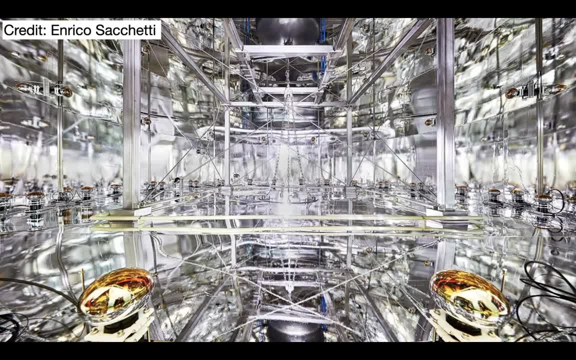 any machine that you build to detect dark matter, right? So if a dark matter particle can go through atoms, any machine or detector you build to try and catch dark matter is also going to be made of atoms. So dark matter can just happily go through the machine and out the other side. 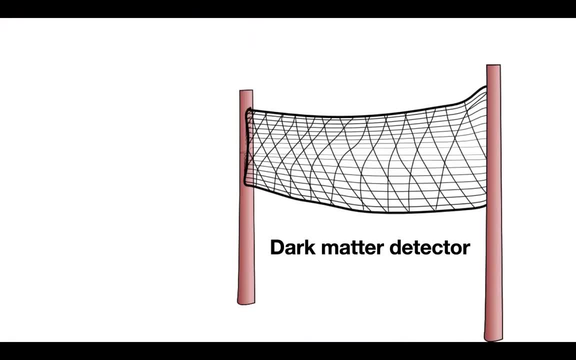 and you're not going to find anything. It's a bit like you know. an easy way to explain it is: you're building a dark matter detector, which is like a net that you want to catch some dark matter in, And then dark matter particles are like tiny, tiny things that are much, much smaller than the. 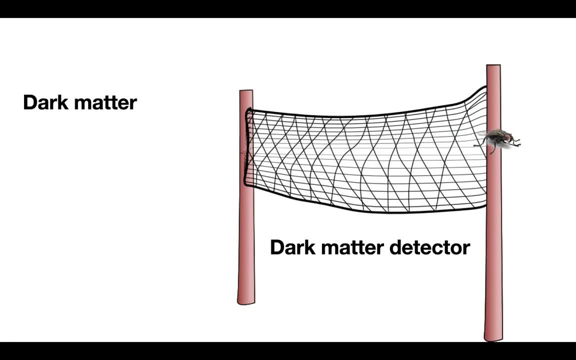 holes in the net, right, Like trying to catch a fly in like a tennis net or something. It can just happily go through the holes and you can't catch anything. So that's what's happened so far. right, We've built these dark matter detectors, but so far they just haven't been good enough. The holes, 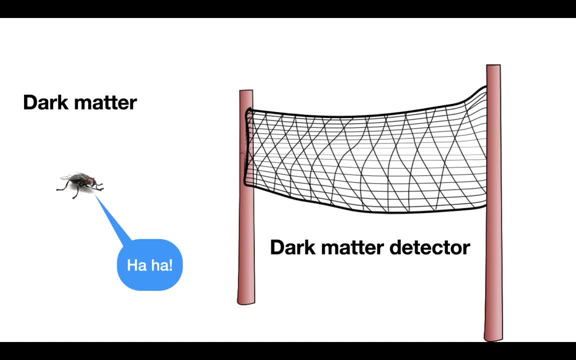 in the net have not been small enough to catch a particle of dark matter, And so what we're trying to do is we're trying to build better and better dark matter detectors, make the holes in the net smaller and smaller, So eventually we're hoping we can catch one of these particles, but it's very 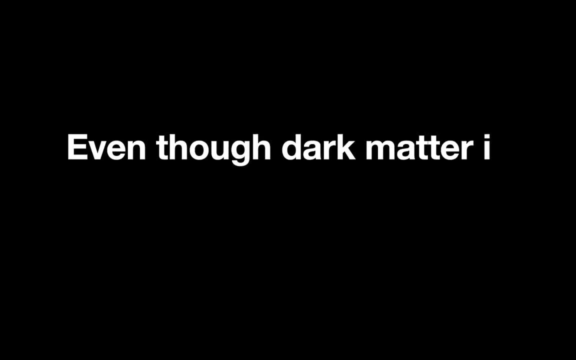 very difficult, Then we haven't been able to do it so far. So, even though dark matter is very strange, and even though we don't know that much about it- because we've never been able to catch one of these particles- we don't really know what they are, But what we do know is that dark matter 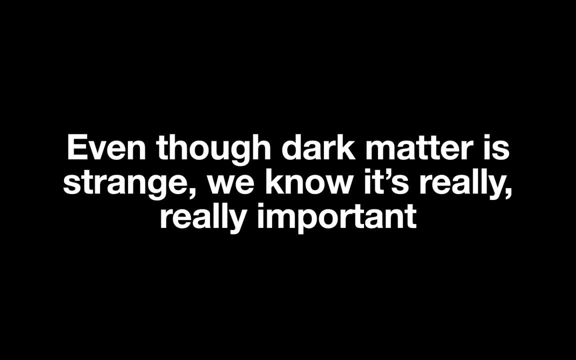 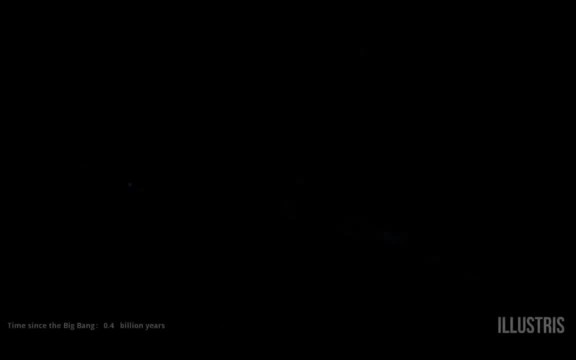 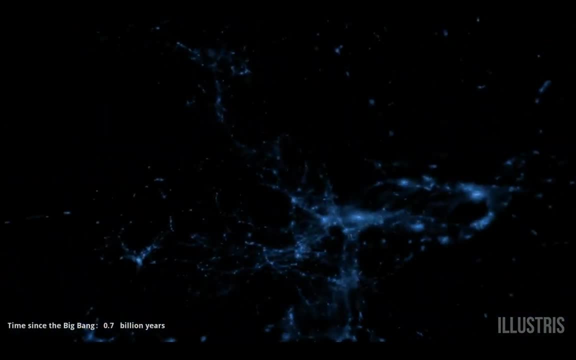 is really, really important, Because if it wasn't for dark matter, the universe as we know it would not exist. So this is a simulation of a universe. This is a toy universe that astronomers build inside a computer. So this is a program called Illustris. It's a model universe running. 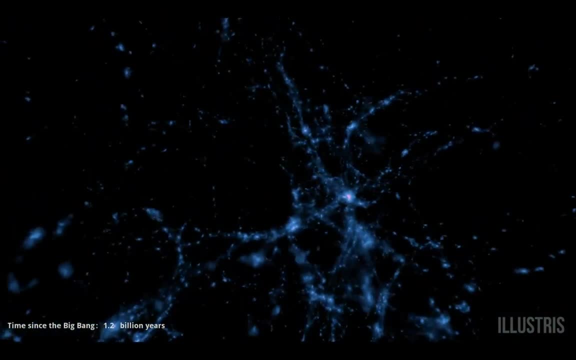 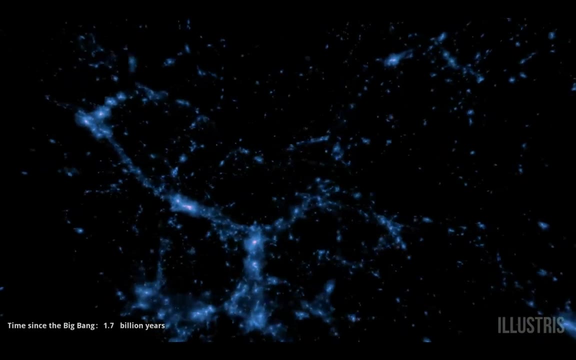 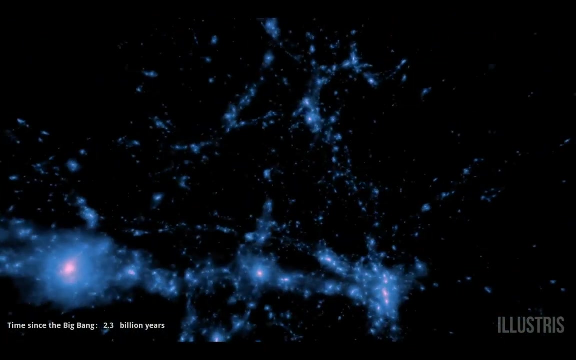 inside a supercomputer And all of the blue stuff you can see here is dark matter, And this is a really, really big chunk of the universe. Every tiny little speck is like a galaxy And all of, And what we've worked out from our models of the universe is that if you don't have dark matter, 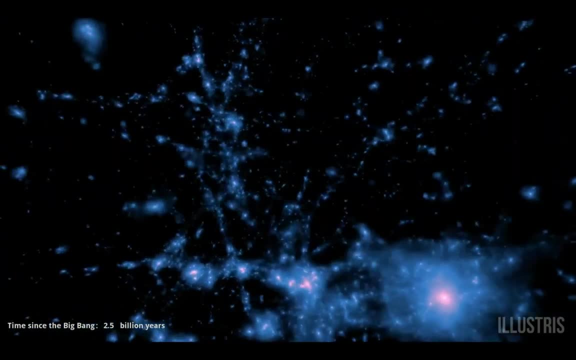 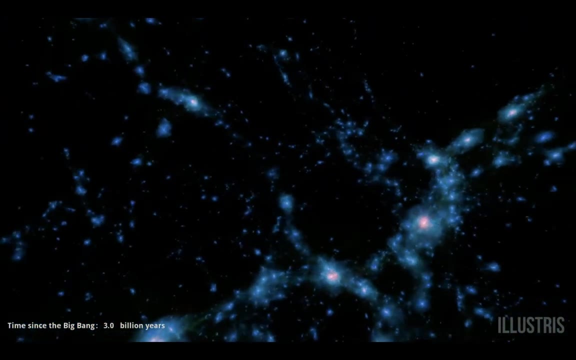 the universe as we know it doesn't form Like dark matter, provides like the skeleton of the universe, if you like, or the scaffolding of the universe. So dark matter kind of clumps together and forms structures And then the rest of the universe, what we think of as the real universe. 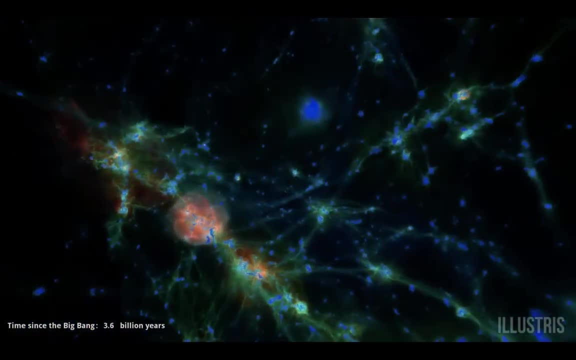 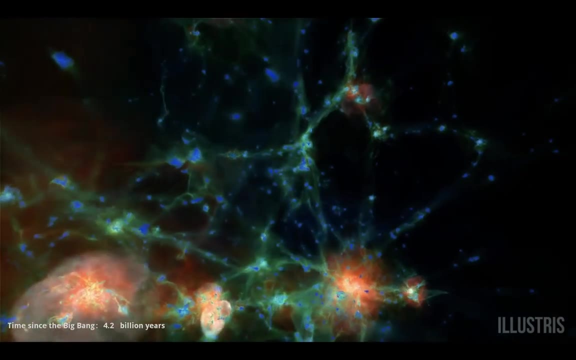 forms around it. Dark matter comes first and provides the scaffolding for the entire universe. So when we look around and we see planets and stars and the planet that we're living on, galaxies out there in space, none of it would exist if it. 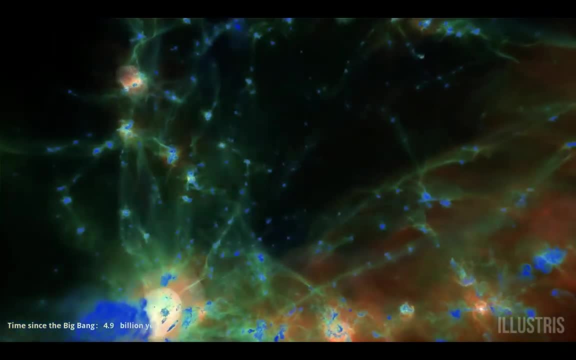 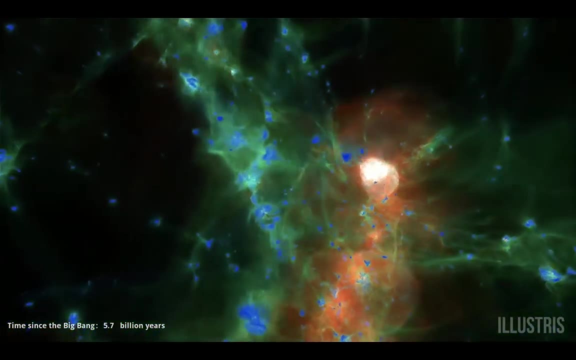 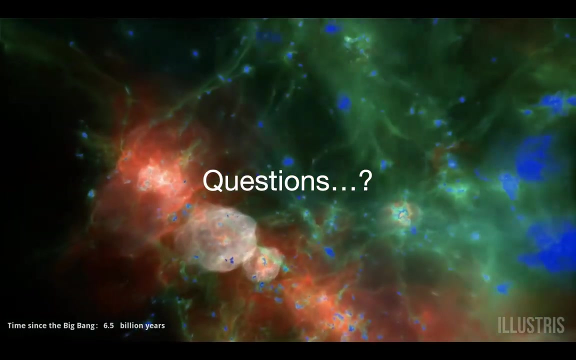 wasn't for dark matter. So, even though this stuff is very, very strange and very, very spooky, it's really, really important. It's only because of dark matter's existence that the universe as we know it exists at all, which I find absolutely amazing. Okay, I think. so that is a good place to 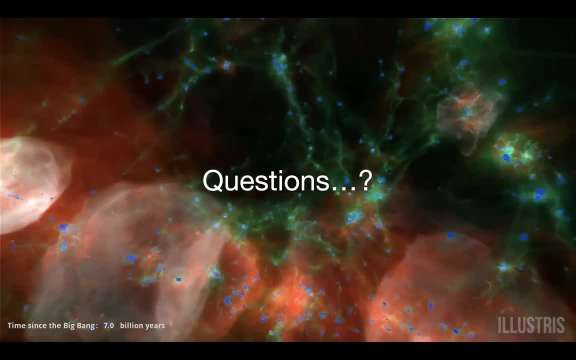 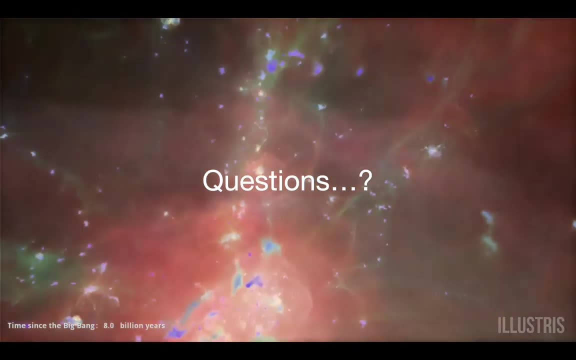 end. So dark matter very, very interesting. We know it's there. We don't know what it is, but we do know it's very, very important, And the universe only exists because of dark matter. So what I want to do now is switch over. 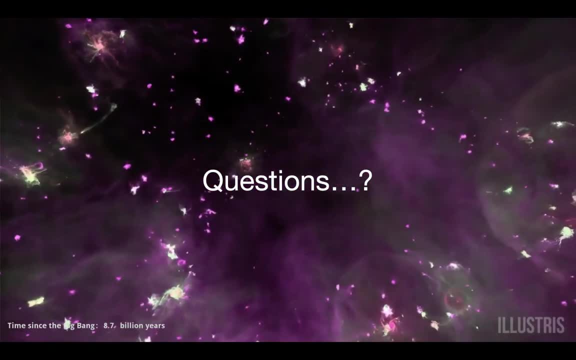 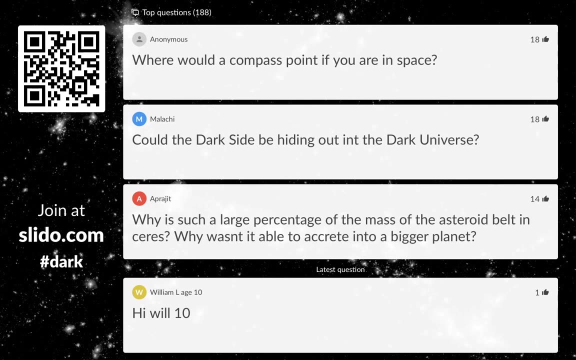 to some of your questions. Where are we? Here we go, Okay question oh 188 questions. I'm going to do my best to answer a few of these. We've got about kind of 15 minutes or so, Okay, so where anonymous ask top question? 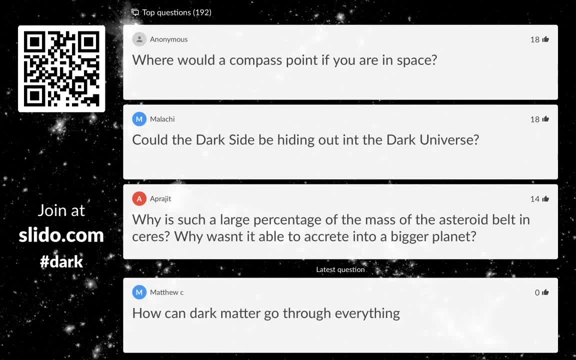 where would a compass point if you are in space? So most likely a compass wouldn't do anything if you're in space. So what compasses on Earth do is follow the magnetic field of Earth. So the needle of the compass points to the north of Earth because 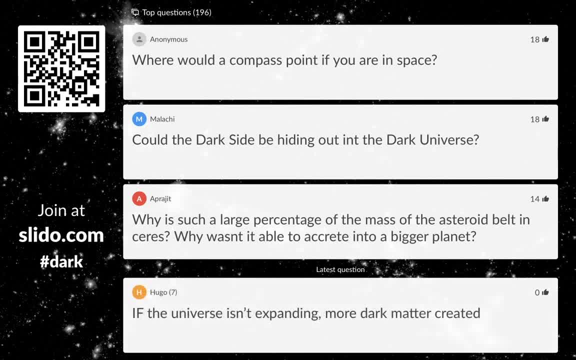 it's being manipulated, it's being moved around by Earth's magnetic fields. There are magnetic fields in space, but generally they're much, much, much weaker than when we are, than when you're near a planet, Because being on the surface of a planet 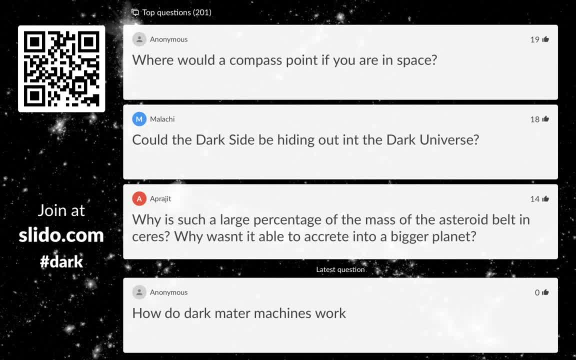 we are next to a big ball of iron. right The Earth's core is made of iron. We're basically standing on a big magnetized ball of iron. So the magnetic field right here is stronger than in most places in space. So generally, if you're in space, 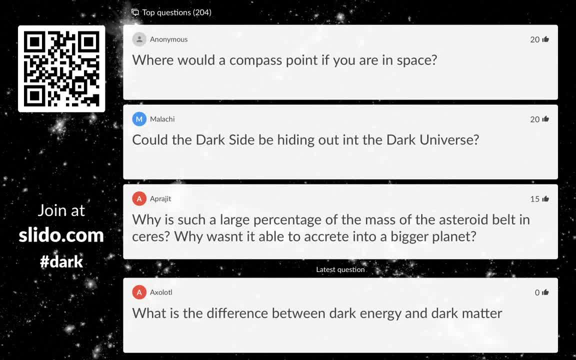 a compass just wouldn't point anywhere because the magnetic field is not strong enough. But if you are close to something with a very strong magnetic field, like stars have magnetic fields, or neutron stars, pulsars have very, very strong magnetic fields, And if you were near one of those, then the compass would point towards. 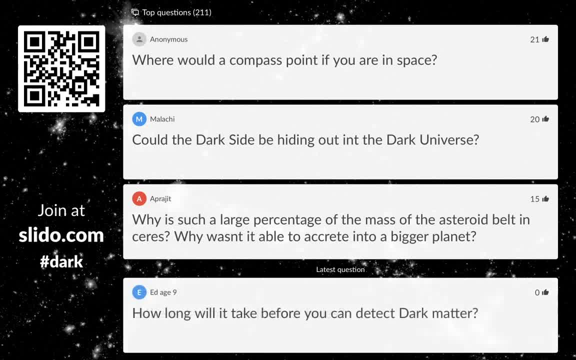 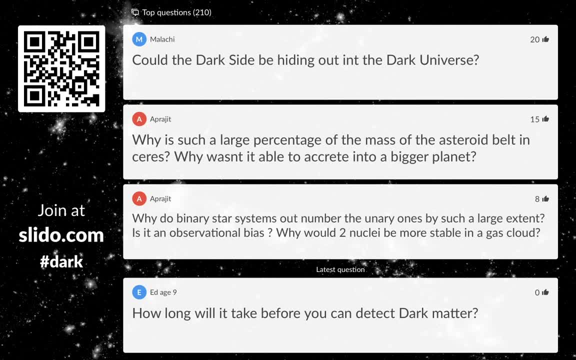 uh, the thing with the strong magnetic fields. Malachi says: could the dark side be hiding out in the dark universe? Uh, I don't know if what you mean by the dark side. I don't know if you mean dark side in some kind of Star Wars way, but it is the idea of there being this dark universe is interesting. 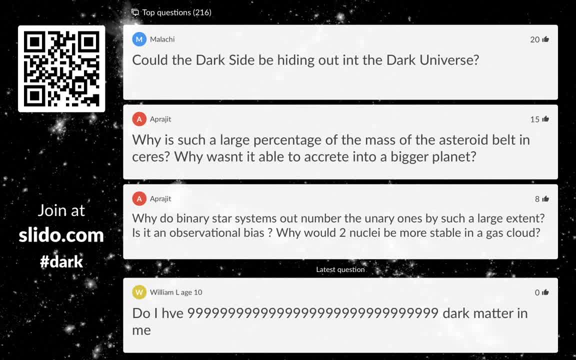 So one idea is that there might actually not be just one kind of dark matter. There might be a whole range of dark particles, There might be a whole dark universe out there, made of all different things that we can't uh, quite detect. Uh, so right now, almost any question about the dark universe, one of the the answer has to be: 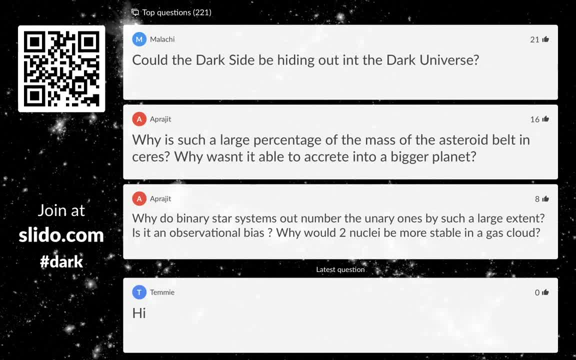 we don't really know yet. We're doing our best to find out about dark matter. We know little bits about it. We know what it does, We know how it forms our universe. Uh, but what dark matter actually does? we'd like yeah. 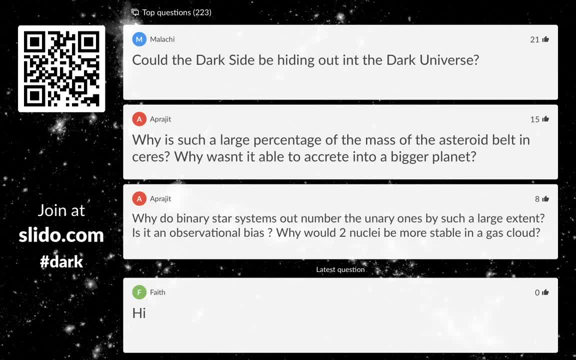 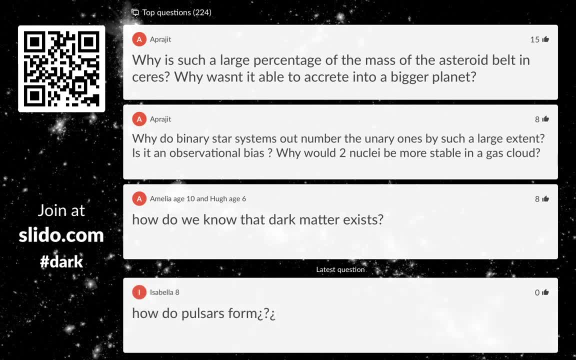 there's lots of mysterious things so far. Great question I bet I could answer. I wish I could answer better. Uh, Aperjit asked a couple of fantastic questions. Uh, so first of all, why is such a large percentage of the mass of the asteroid belt? 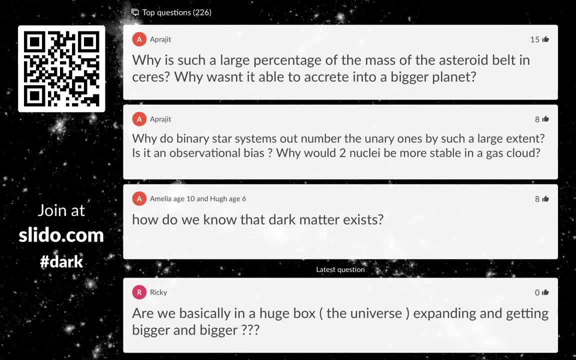 Uh, so, first of all, why is such a large percentage of the mass of the asteroid belt and Ceres? why wasn't it able to accrete into a bigger planet? Uh so, the asteroid belt, of course, this ring of rocks in our solar system between Mars and Jupiter, and uh the and Ceres, is the the biggest thing in the asteroid belt. 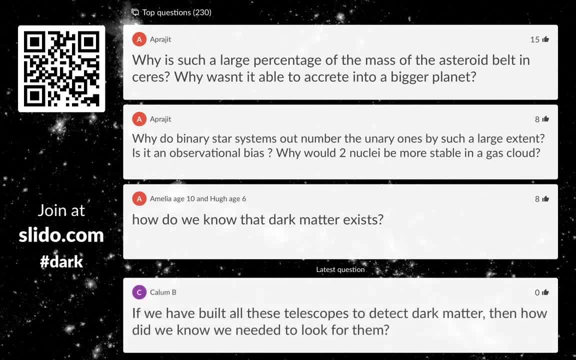 Uh, the, even still the. the asteroid belt taken as a whole isn't actually that heavy. If you add up the entire asteroid belt, so not just Ceres but all the other stuff as well, you would only get to about 10% of Earth's mass. 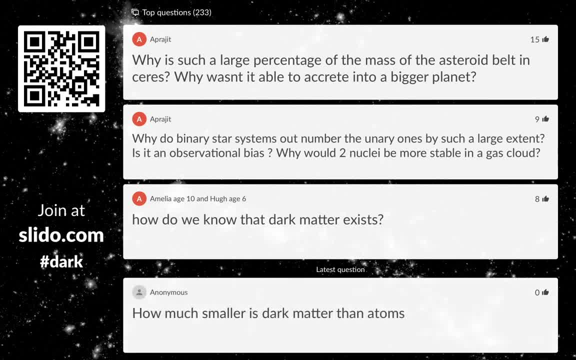 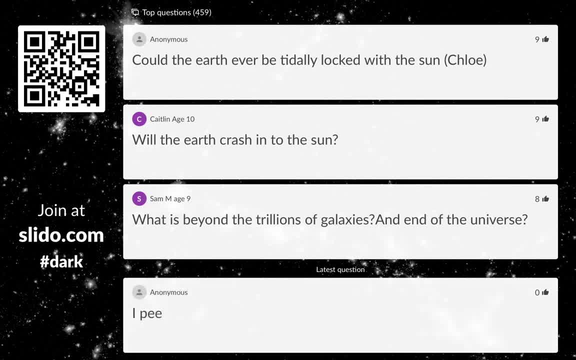 Uh, but we think the asteroid belt couldn't coalesce is because of the mass of the asteroid belt. Uh, but we think the asteroid belt couldn't coalesce is because of the mass of the asteroid belt, Uh. so for anyone that doesn't know what being tidally locked is, 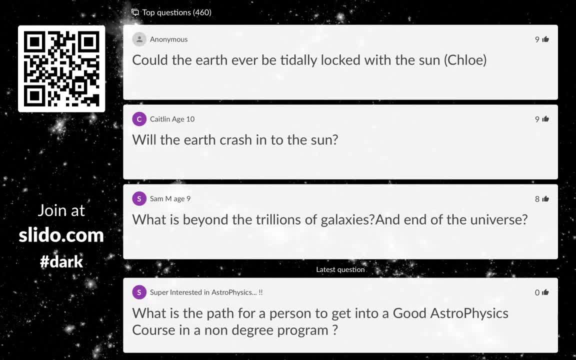 Um, if two things are orbiting quite close together, Um, they can end up that the time you take to complete one orbit is the same as the time you take to spin around once, And when that happens, you end up having the same face pointing towards the thing at all times. 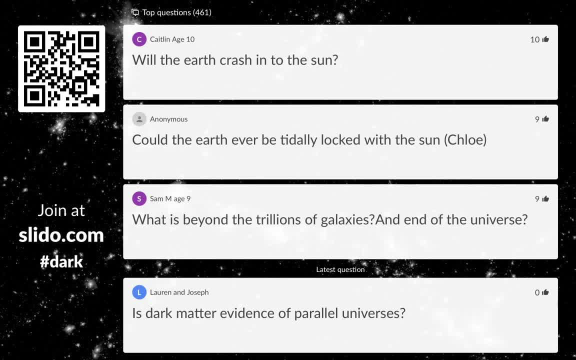 So a really easy example of this is that the moon is tidally locked with the Earth, right? That's why we see one side of the moon all the time, and then there's the dark side of the moon on the other side That we don't see. That's because the moon is tidally locked with the Earth. Um, it would be very sad if the Earth became tidally locked to the Sun, because it would mean there'd be no more day and night and one side of the world would be in permanent daylight. 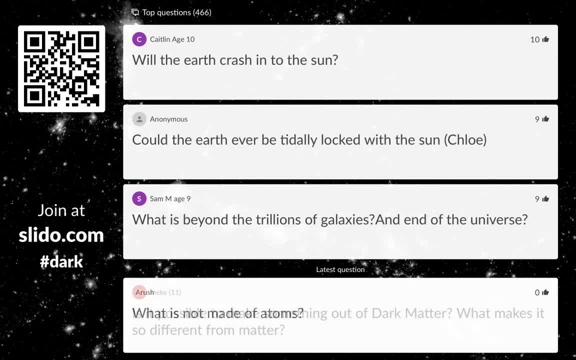 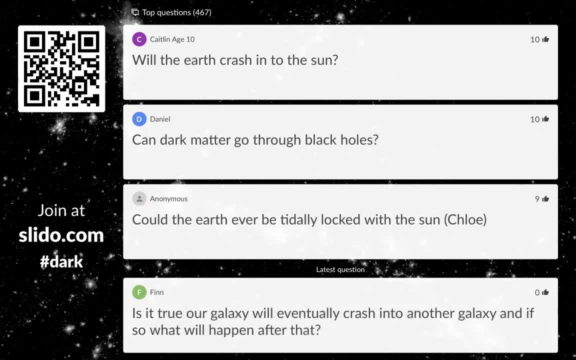 and one side of the world would be in permanent nighttime, or at least until you waited half a year and we- uh, they swapped around. Um, so luckily for us, the Earth is not going to be tidally locked with the Sun. 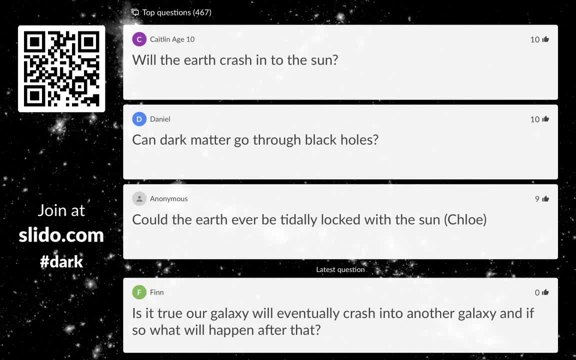 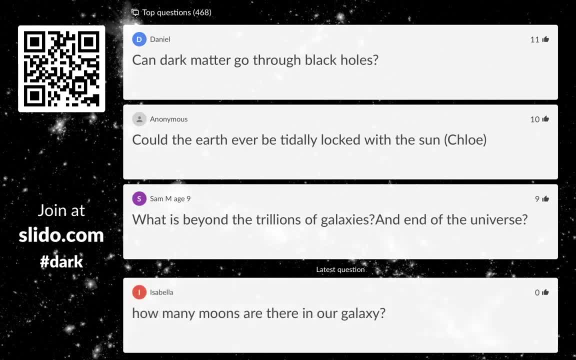 We are just too far away. So, yes, very happy to say that that won't happen. We are going to continue to have days and nights for the future. Uh, where are we? Uh, can dark matter go through black holes? 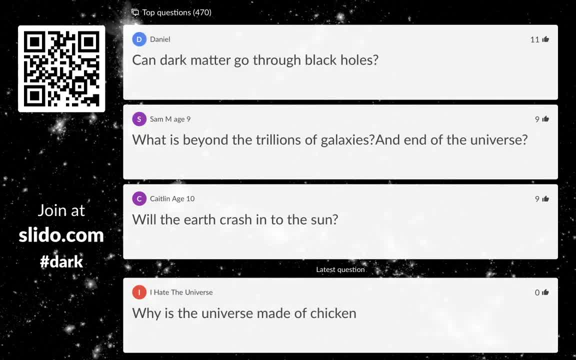 Uh, so first of all, I think, uh. so I spoke about dark ho-, about black holes, last week. If you didn't catch that, you can find that on our YouTube. Uh, things don't go through black holes. 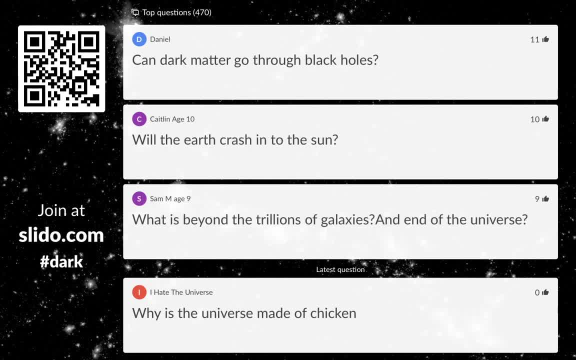 Black holes aren't portals. Uh, they are just, uh, they are. they are just kind of dots in space with very strong gravity that can swallow things, Uh. but dark matter can get swallowed by black holes, uh, just as much as regular matter. 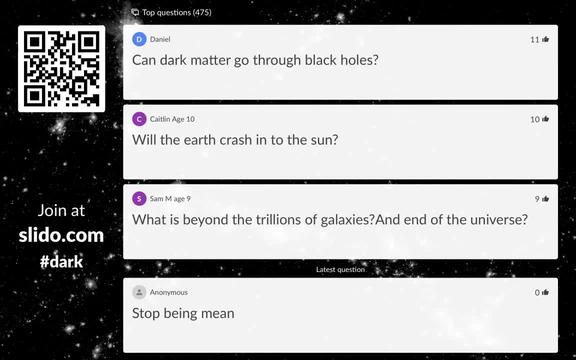 Uh. Caitlin says: Will the Earth crash into the Sun? Uh, again, I'm very happy to say that the answer is no. Uh, our Earth is just going to happily continue orbiting the Sun for thousands of millions of years to come. 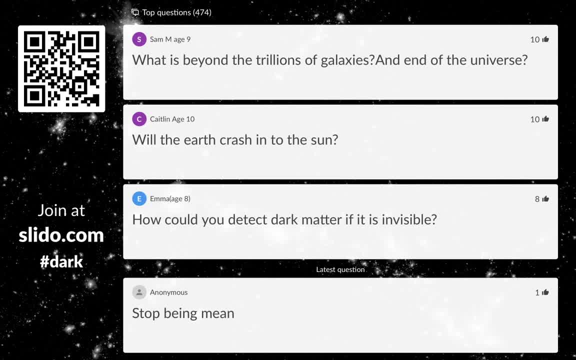 Eventually, uh, in about 5,000 million years' time, the Sun, uh, is going to reach the end of its life and swell up, and then we'll probably- and so the Earth will- crash into the Sun, then, not because we've fallen in.